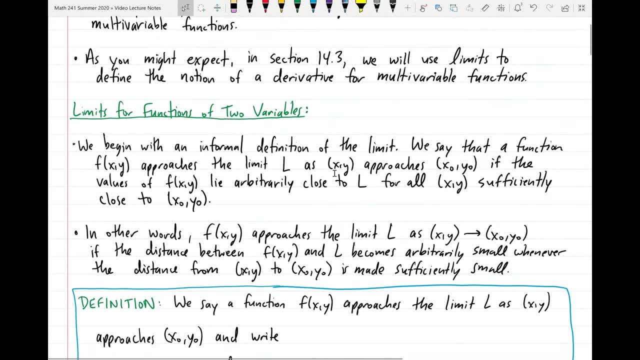 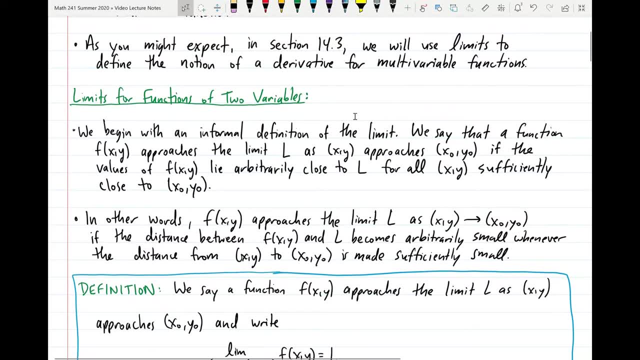 used the limit to define a derivative, So we're going to use the limits that we define in this video to define a derivative. Okay, so let's move on to limits for functions of two variables. So I'm going to start off by giving an informal definition of the limit and I'm going to rephrase the idea. 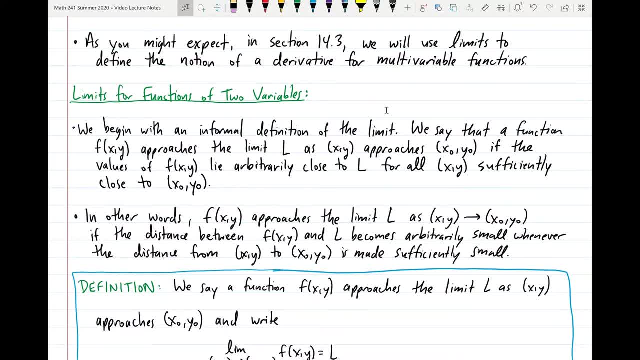 of the limit multiple times here, just to try and build up an intuition of what the limit is, apart from the rigorous definition. Okay, so for the informal definition we say that a function of x- y approaches the limit L, where L is just some real number here, as x- y approaches the point. 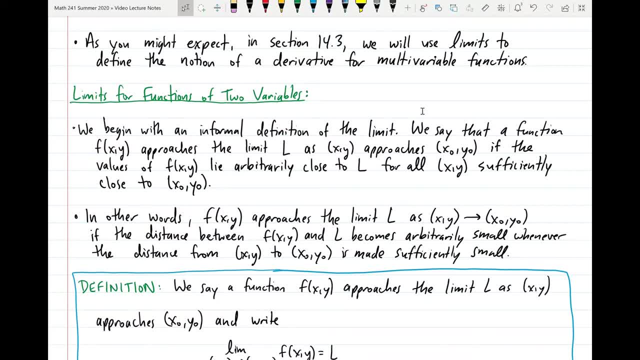 x-naught y-naught if the values of f of x, y lie arbitrarily close to L for all points x, y sufficiently close to x-naught y-naught. If you need to, you can pause the video and read through. 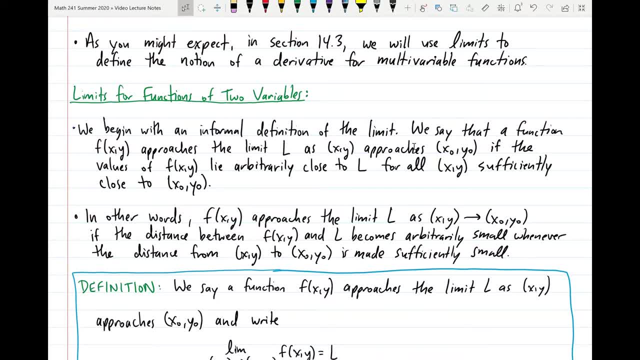 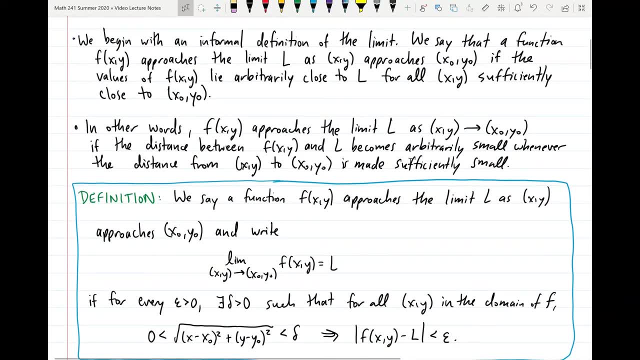 that a couple of times. but that is the kind of informal idea of what a limit is. So, for example, f of x? y approaches the limit L as x? y goes to x-naught y-naught if the distance between f of x, y and L becomes arbitrarily small. whenever the distance from x? y to x-naught y-naught is made sufficiently small, 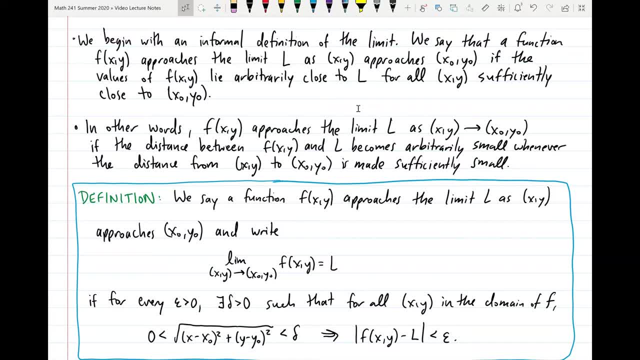 So there's a way of just rephrasing the informal definition that I gave. There will be another informal definition a little bit further down. that, I think, is the most intuitive, but that's the way that we're going to cap off the discussion of limits. 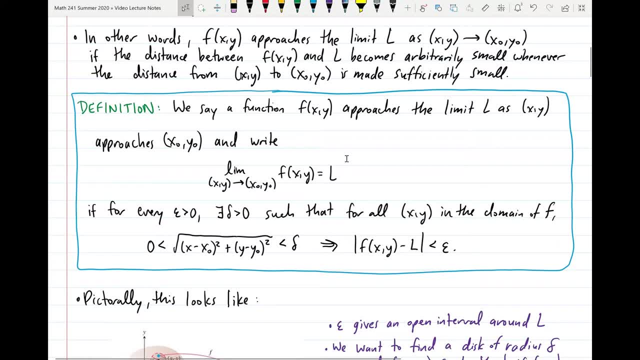 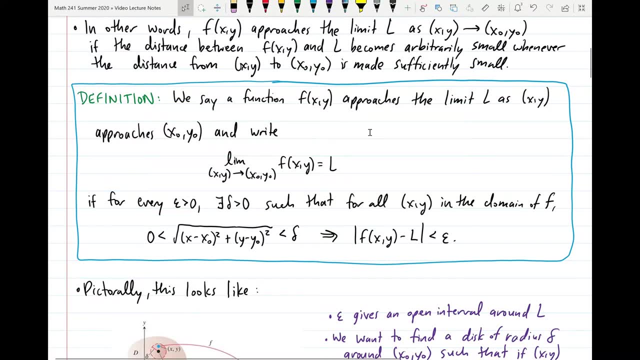 So now here's the technical definition of what a limit is. This is the definition that you have to appeal to if you want to prove that some real value, L, actually is the limit. as x, y approaches, x-naught, y-naught for some function, f. So we say: 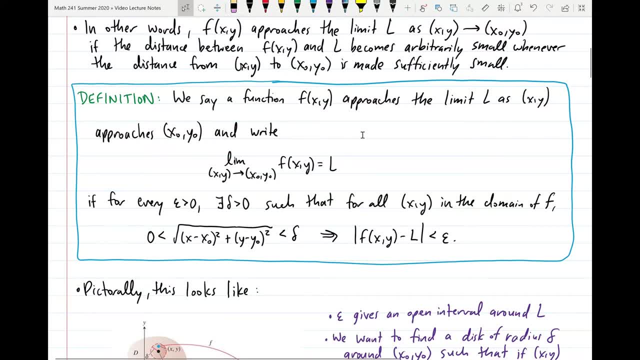 a function f of x- y approaches the limit L as x y approaches the point x-naught, y-naught and write limit as x y goes to x-naught, y-naught of f of x- y is equal to L If for every epsilon: 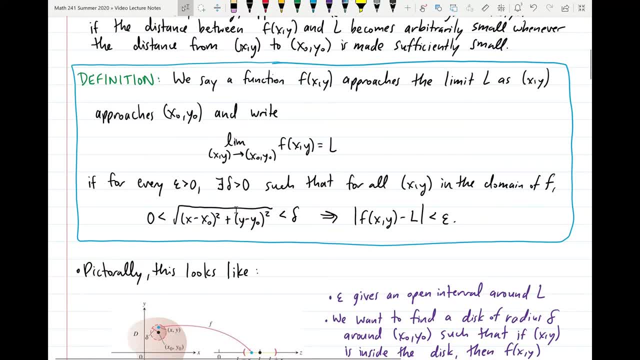 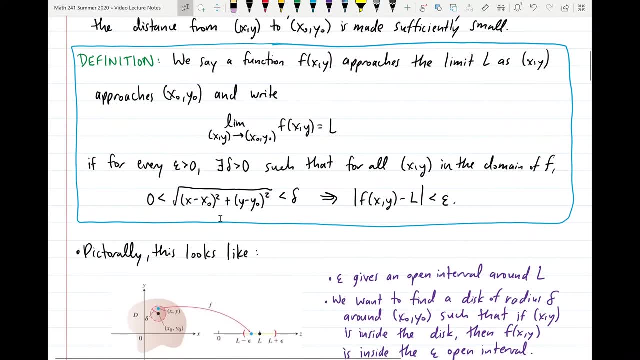 greater than zero. there exists a delta greater than zero, such that for all x, y in the domain of f, if the square root of x minus x-naught squared, plus y minus y-naught squared is greater than zero and less than this, 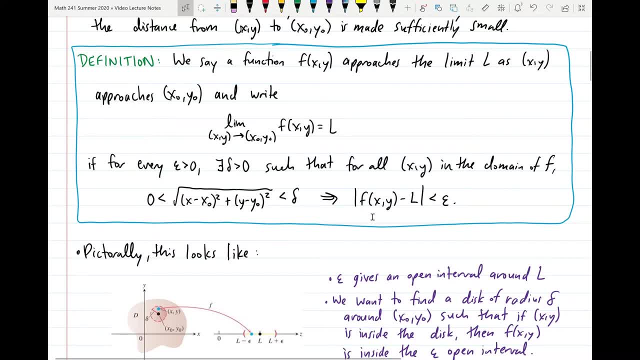 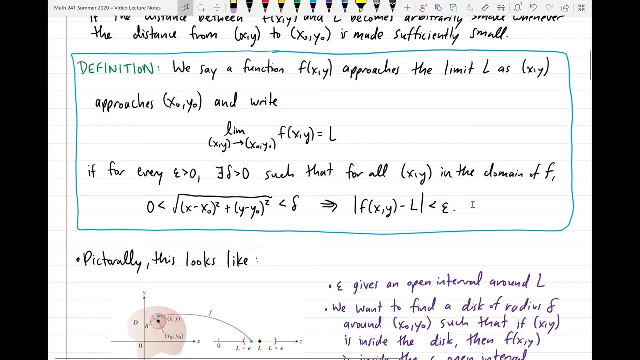 delta that we picked. then it implies that the distance from f of x, y to L is less than epsilon, or the absolute value of f of x, y minus L is less than epsilon. And again, I know that this definition is quite a monster to cut to try and understand in your mind. 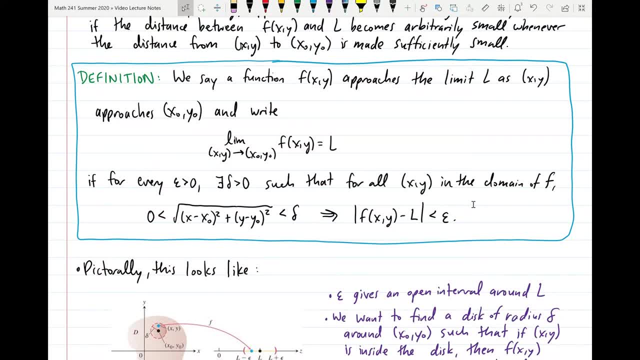 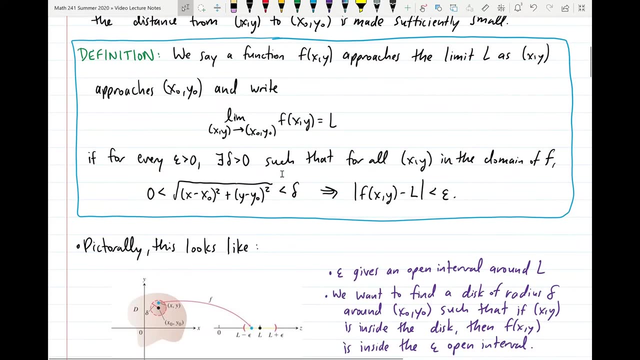 but hopefully we can make a little bit more sense of it as we go throughout this video. I do want you to notice that the definition is just a generalization of the same epsilon delta definition that was given for single variable functions in calc 1 and calc 2.. The difference here is that we have to define 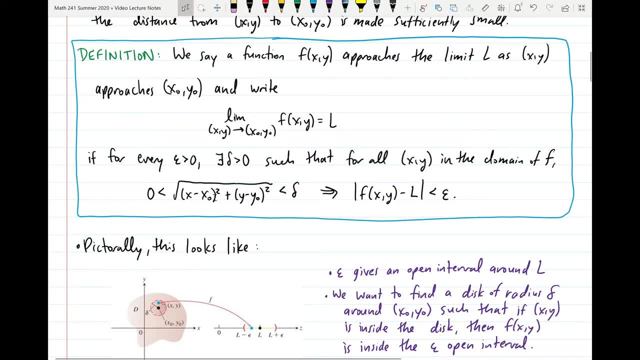 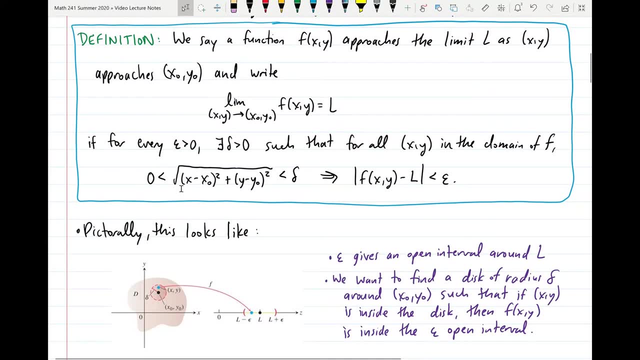 the distance between points in the plane differently than the distance between real numbers on the number line. So the fact that the square root of x minus x-naught squared plus y minus y-naught squared is greater than zero and less than delta means that the distance from the point x y to the point x-naught. 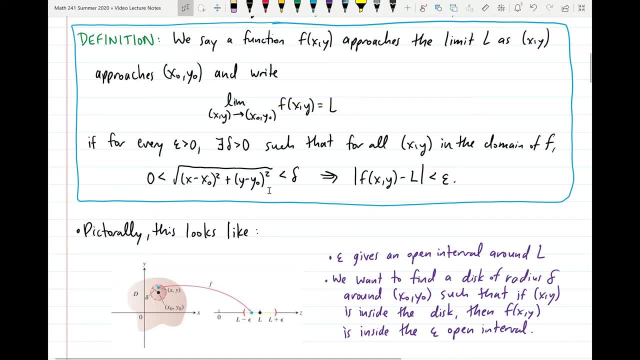 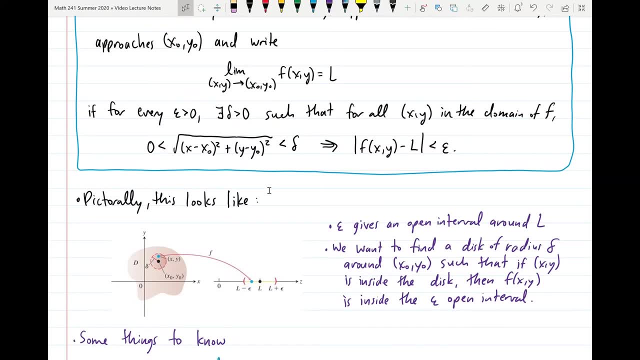 y-naught is greater than zero and less than delta. So we are we're using a different notion of distance between points, But other than that, the definition is really the same as it was for calc 1.. So now let's give a little bit of a look at the definition of the point x, y and less than delta. 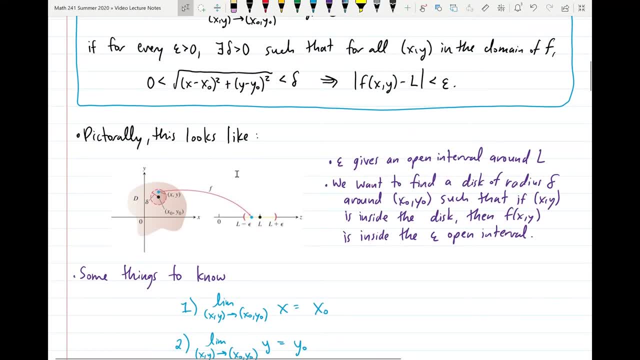 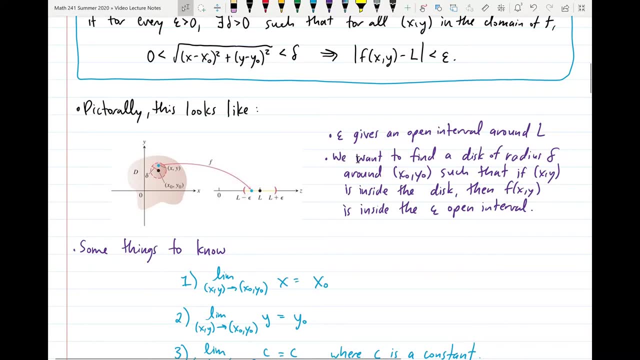 So now let's give a pictorial description of what this definition is really saying here. So if we pick some epsilon greater than zero, then that epsilon around the limit L is going to give us this open interval which is over here, this open interval made with the red parentheses on. 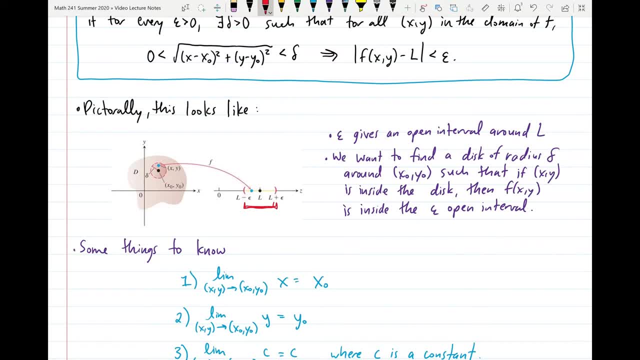 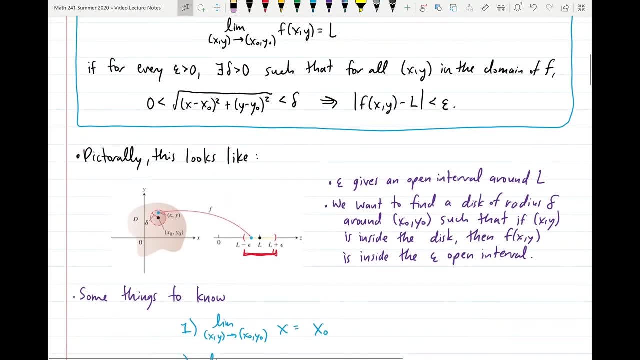 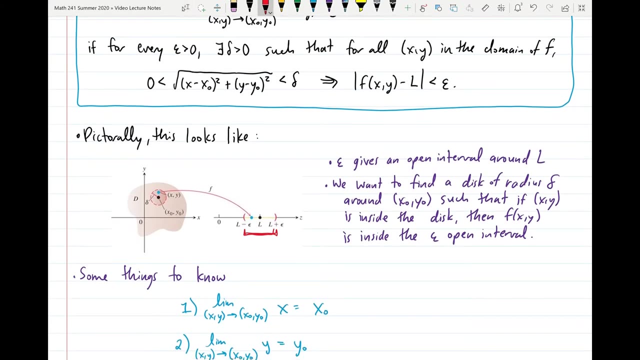 the number line. So that's what happens after we pick some arbitrary epsilon greater than zero. And to show that the limit exists and that the limit is L, we want to find a disc of radius delta that contains the point x-naught- y-naught. So x-naught- y-naught is the point we are limiting to. 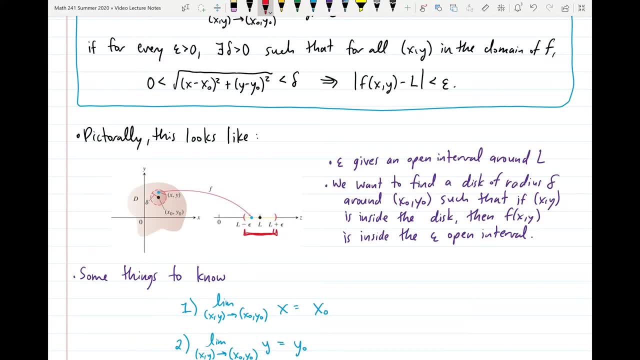 And we want to find a disc of radius delta centered at that x-naught, y-naught, such that if we take any point x, y, so in the diagram here we have that point x, y and blue. If we take any point x- y inside of that disc and send it through the function f, 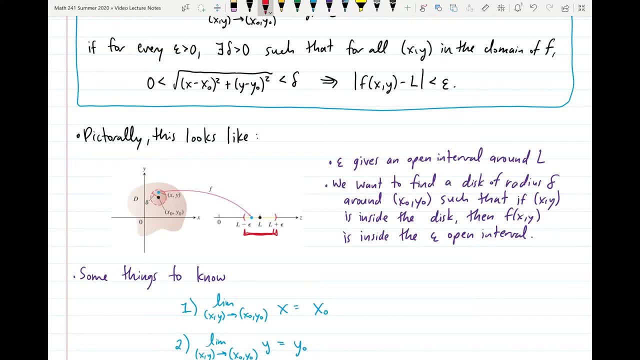 then that point is going to map inside of that epsilon interval on the line. So let me say that again, We want to find a delta such that if we make a disc of radius delta centered at the point x-naught, y-naught, and we take any point- x, y inside of that disc, then when we map it through, 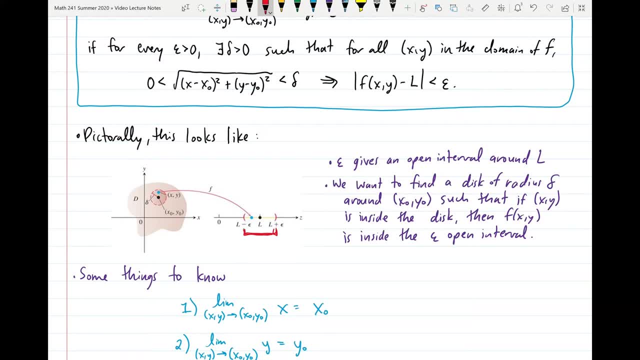 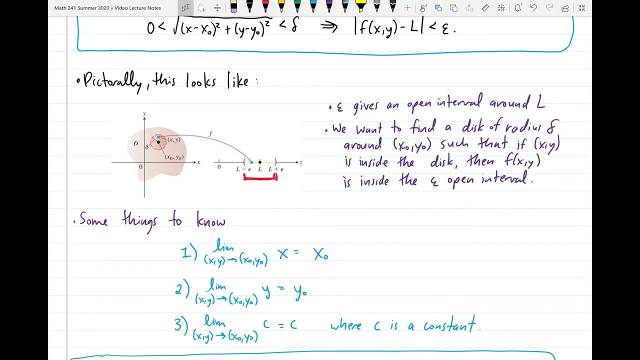 the function f, it's going to map inside of that open interval made by epsilon. So I think this is the most intuitive way to think about it. We're trying to find a space that is small enough around the point x-naught, y-naught, such that all of the points inside of that space 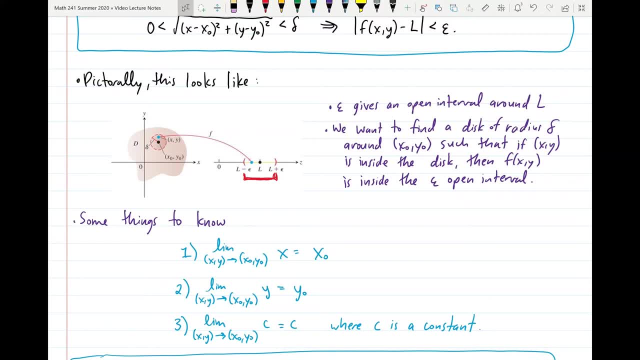 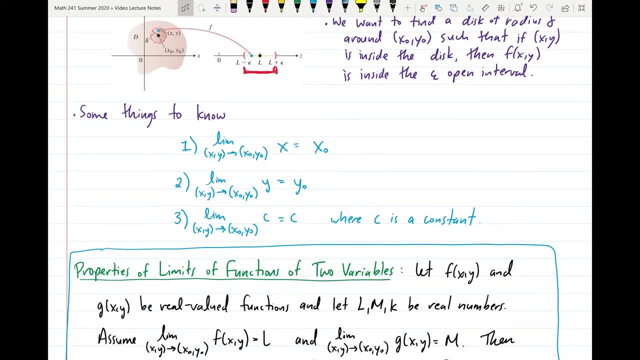 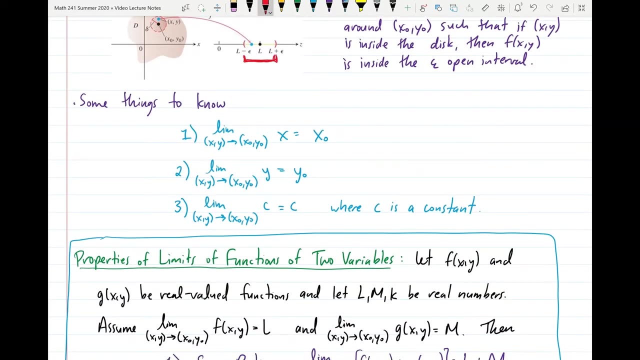 map inside of that space, inside of the epsilon space, on the real number line. So here are some things to know about these limits of functions of two variables. So, first off, if we just have the function x, then the limit, as x, y goes to any point, x-naught, y-naught is going to be equal to x-naught And the same can. 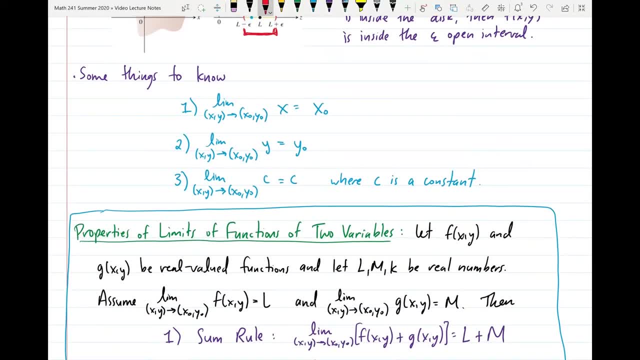 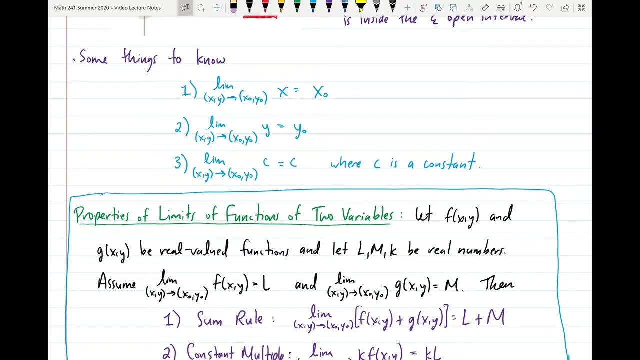 be said about the function y. So the limit as x y goes to x-naught, y-naught of the function y is just going to be equal to x-naught. And then the last thing that I'm going to list here that we need to know before we go into the 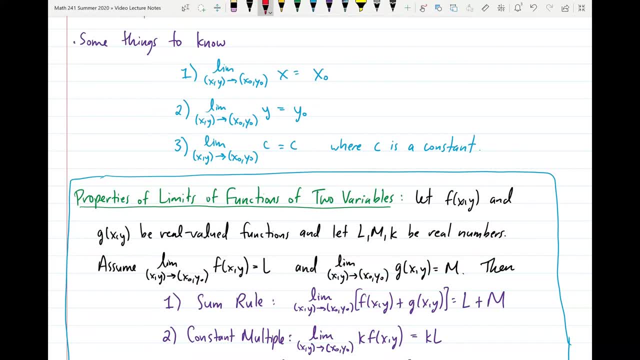 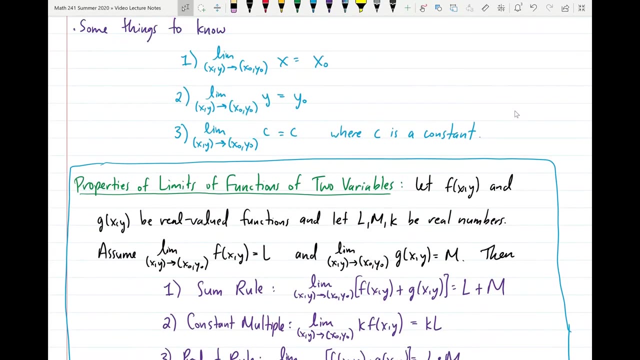 properties of limits below is that if we have a constant function, so the function just maps all points x, y to c, then the limit, as x, y goes to x-naught, y-naught of c, is just equal to c, regardless of what constant c we choose. So now that we've given the definition of the limit, 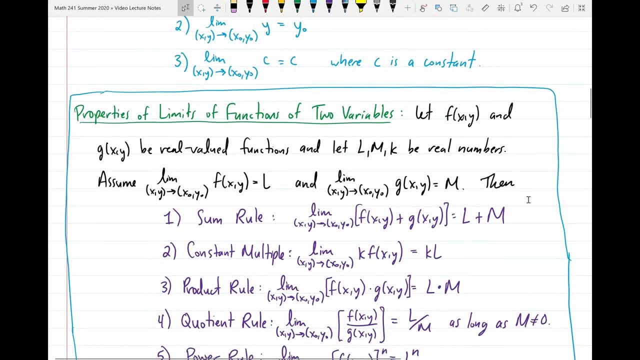 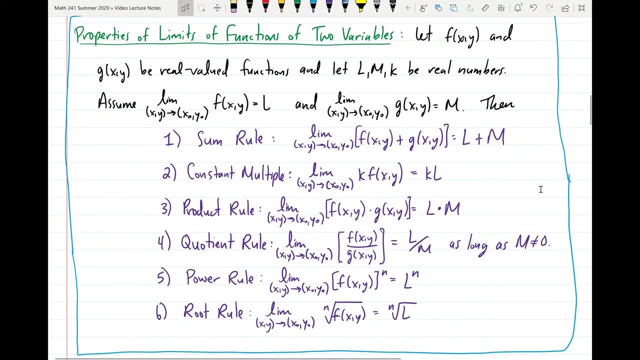 let's start with the definition of the limit. So we're going to start with the definition of the limit. So let's start talking about properties of limits for functions of two variables. So there's a giant list here. I am actually going to go through each one of the properties and just 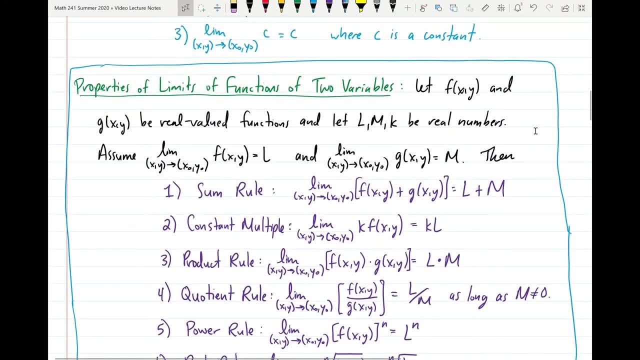 mention it. So if we let f of x- y and g of x- y both be real valued functions and we let capital L, capital M and k be real numbers, and then we're also going to assume that the limit as x. 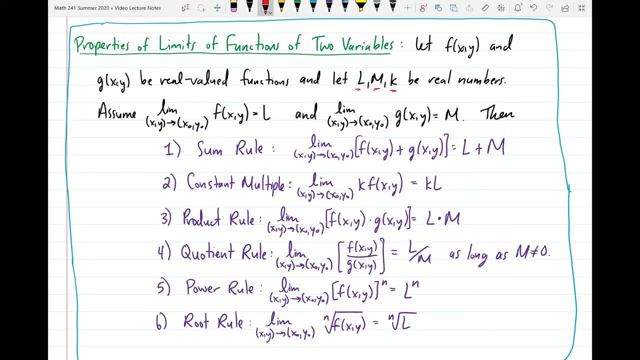 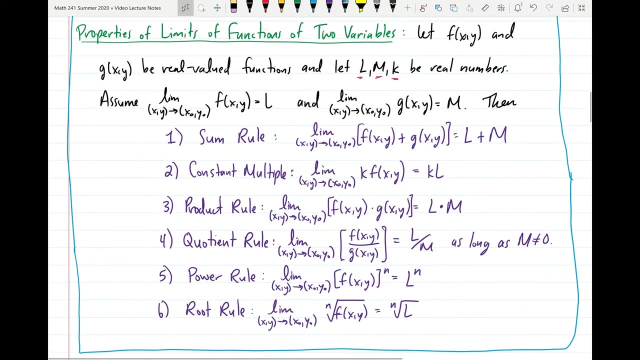 y goes to x-naught, y-naught of f of x y is equal to L, and also that the limit, as the limit, as x? y goes to x-naught, y-naught of g of x y is equal to M. then we have all of these following properties. So the first property is: 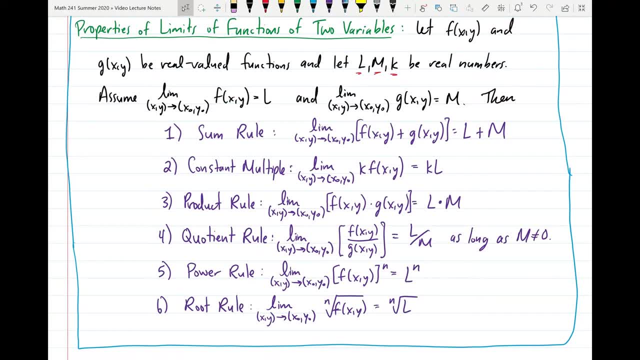 the sum rule and all of these properties ultimately are just generalized from the same properties we had for single variable functions. But we're going to start out with the sum rule. So the sum rule says that if I take the limit of the sum of two functions, then that's going to be equal to the sum of the limits of each. 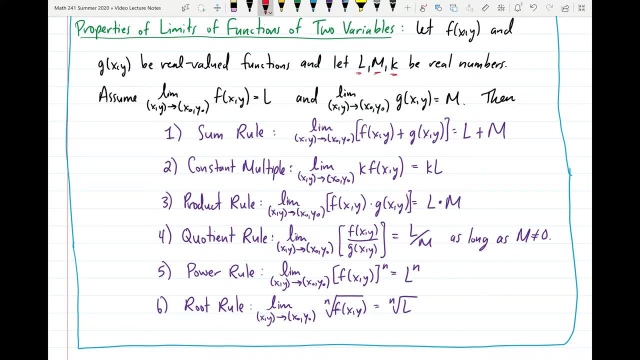 function. So here we have the limit, as x y goes to x-naught, y-naught, of f of x y plus g of x y is equal to the limit of f of x y, which is L, plus the limit of g of x y, which is M. This is: 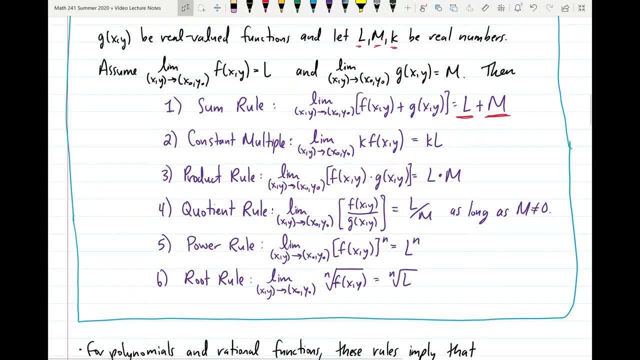 called the sum rule. Okay, the second rule, the constant multiple rule. So if k is just any real number- and I'm going to take the limit of x y plus g of x y, which is L, then that's going to. 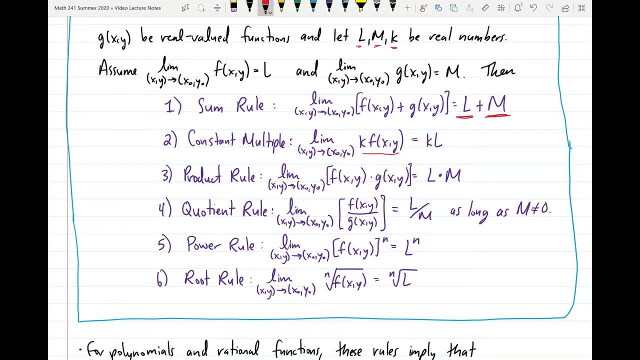 be equal to the sum rule. So if I take the limit of x y and I'm multiplying it by f of x y, then the limit, as x y goes to x-naught, y-naught, of k times f of x y, is equal to k times the limit of f of x y, So k times L. 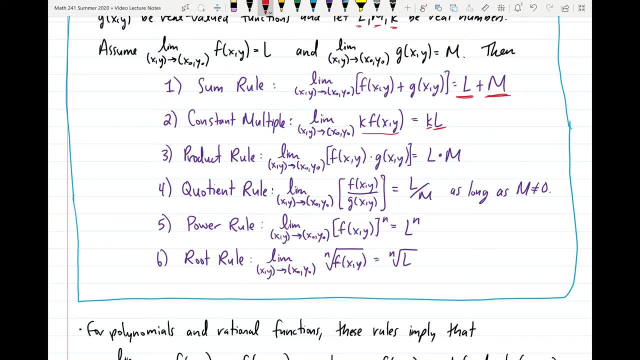 Next we have the product rule, In this case the limit of the product of two functions. so here we're taking f of x- y and multiplying by g of x- y is equal to the limit of f times the limit of g. 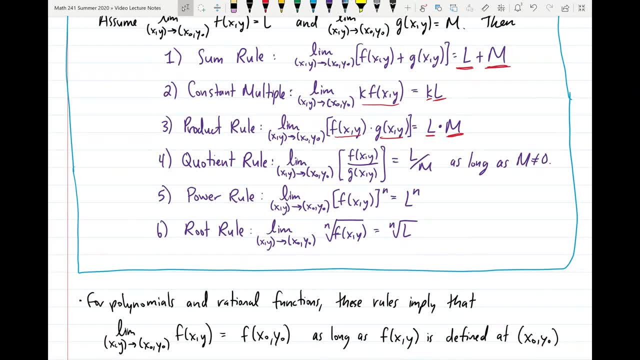 And the quotient rule is very similar to the product rule. If we have f of x- y divided by g of x- y and we want to take the limit of that function, it's going to equal the limit of f of x- y divided. 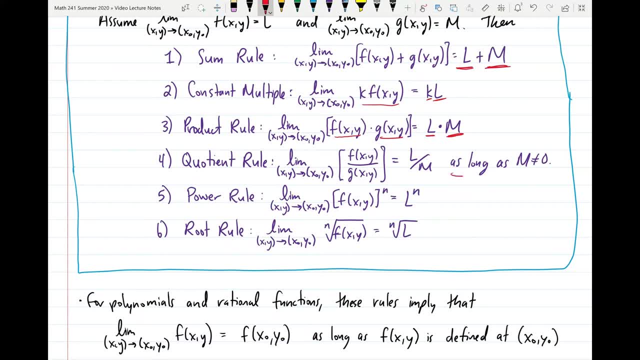 by the limit of g of x- y as long as M or the limit of g of x- y is not equal to zero, Because if that were the case, we'd have division by zero, which is not defined. Next up, we have the power. 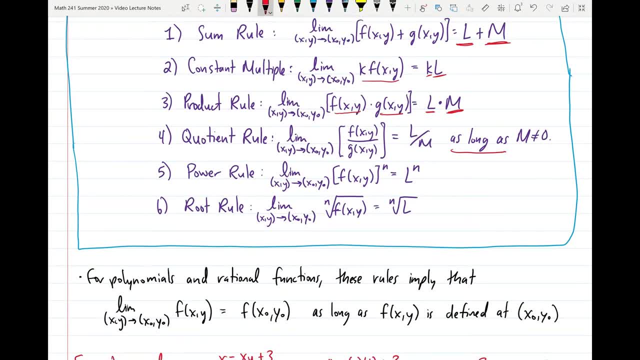 rule which says that if I take my function f of x- y and I raise it to some integer power n, then the limit as x y goes to x-naught, y-naught of that of f of x y to the n is equal to the. 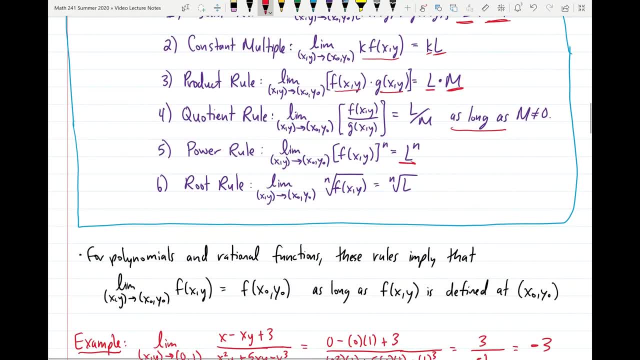 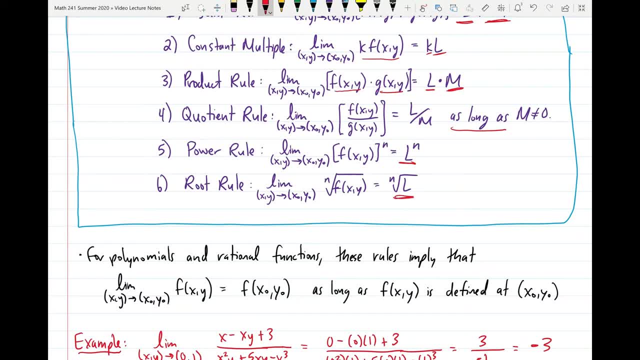 are some conditions that have to be satisfied for the root rule here. So, for example, if n is an even integer, then l is going to need to be greater than or equal to zero. Otherwise we're going to have some kind of square root of a negative number which is not defined for real. 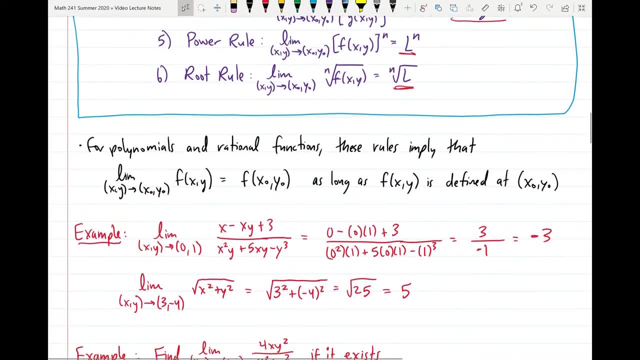 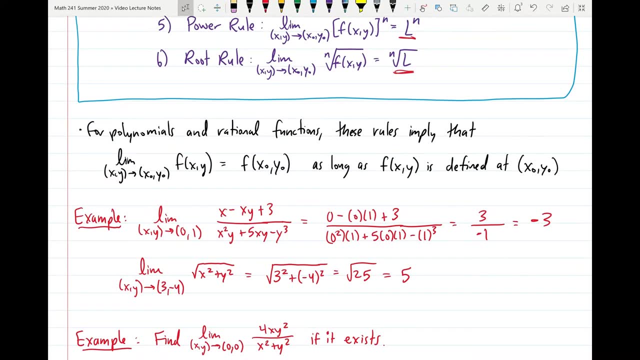 numbers. Okay, and with all of these properties, which I've mostly just listed here for your convenience so that you can reference them, we actually get the following fact: So, if we're for polynomials and rational functions, remember that rational functions are just functions. 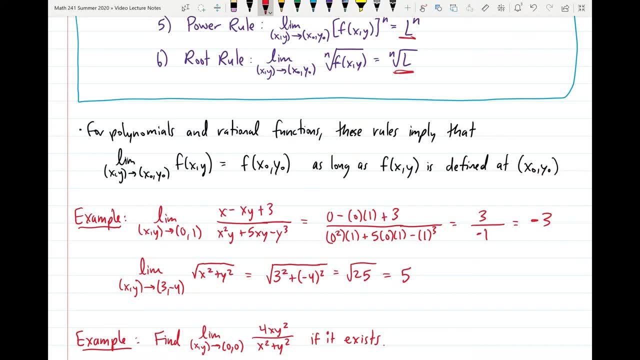 that look like fractions and where the top is a polynomial and the bottom is a polynomial, kind of like the function that I have here in this example. So for polynomials and rational functions, these rules that I just listed above imply that the limit as x, y goes to x. 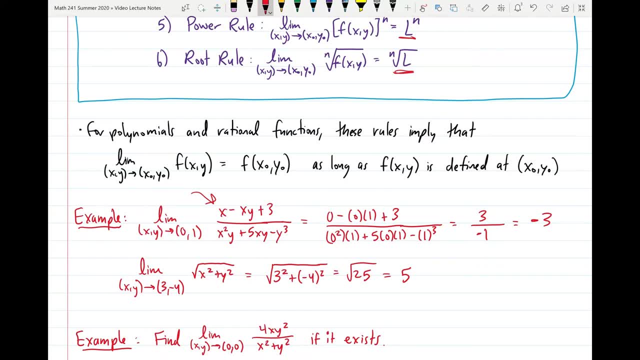 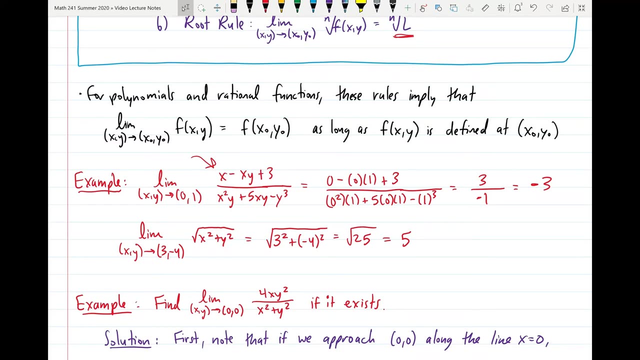 not y, not of f of x, y is equal to f of x, not y naught, as long as f of x, y is defined at x naught, y naught. In other words, remember from calc 1 that if you took the limit of a polynomial or a rational function and you took the point that 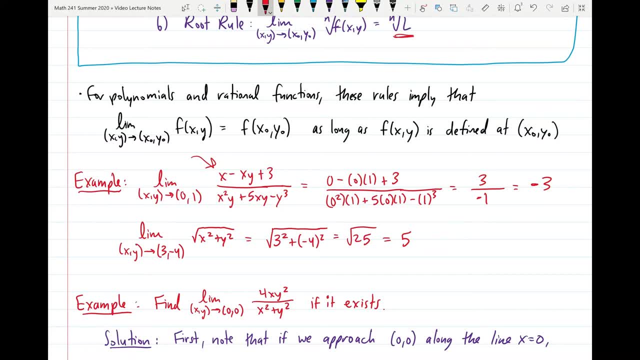 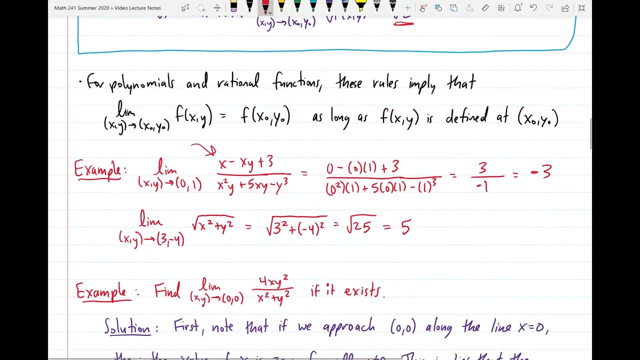 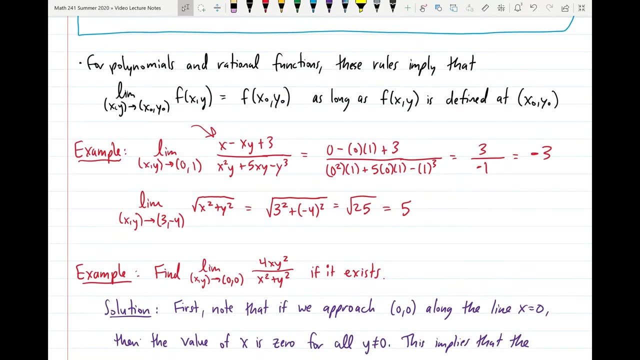 you were limiting to and you could plug it into the function. and if that value that you got when you plugged it in was not zero over zero, as long as it was a determinant form, then the limit was going to equal the value you got when you just plugged it in. So the examples that I have below: 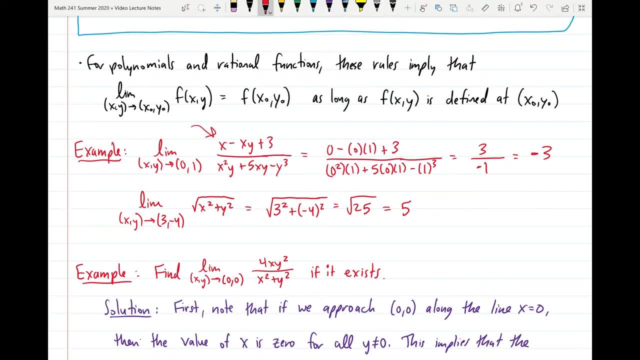 are examples of just that. So first we're going to take the limit as x, y goes to zero, one of the function x minus x, y plus three, divided by x squared y plus five, x y minus y, cubed, and we're going to start off because this is a rational function. let's see what happens if we just plug. 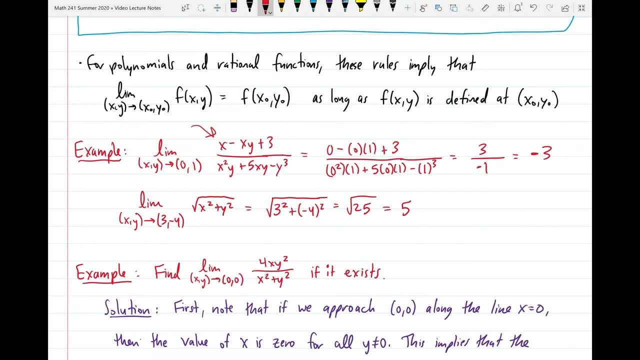 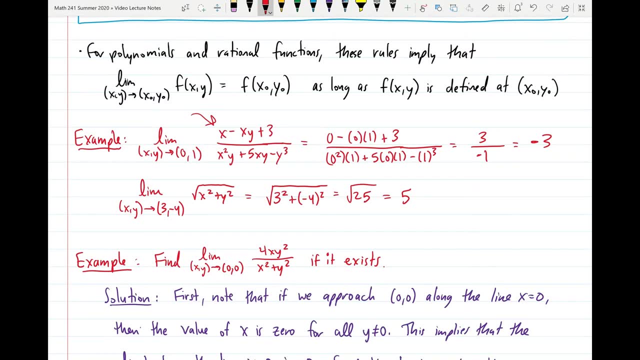 in zero one for our function. What value do we get? So we get a zero one, Zero minus zero, times one plus three over zero, squared times one plus five times zero times one minus one. cubed Again, this is just from plugging in zero for x and plugging in one for y, and if we 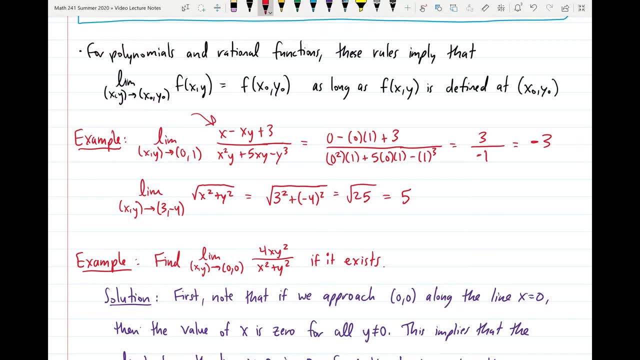 simplify that we get three divided by negative one, which is equal to negative three. So because the function is defined at the point zero one and it's a rational function, then the limit as x, y, goes to zero one. So we're just going to equal whatever value we get when we plug in zero one to our function, which is: 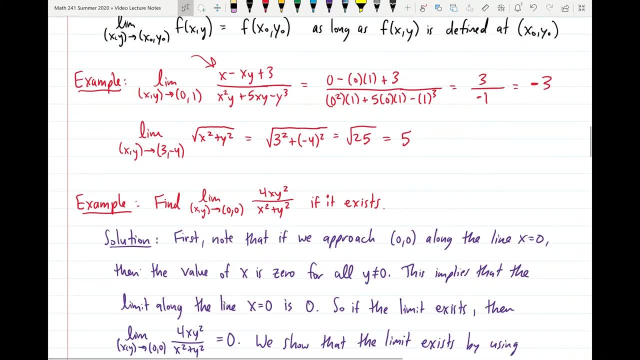 negative three, And then another example of this same concept. So here we have the function is the square root of x squared plus y squared, and we're going to take the limit as x, y goes to three minus four. Then we can start off by just seeing what happens when we plug in three and minus four, for 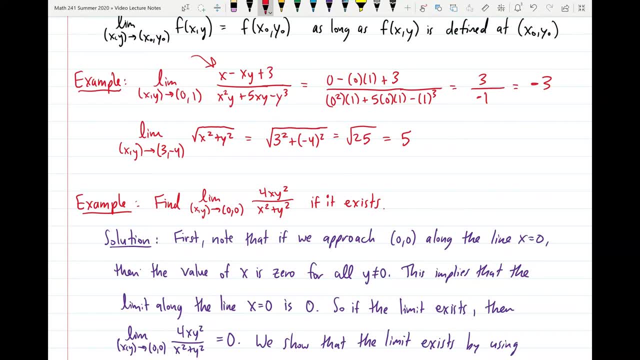 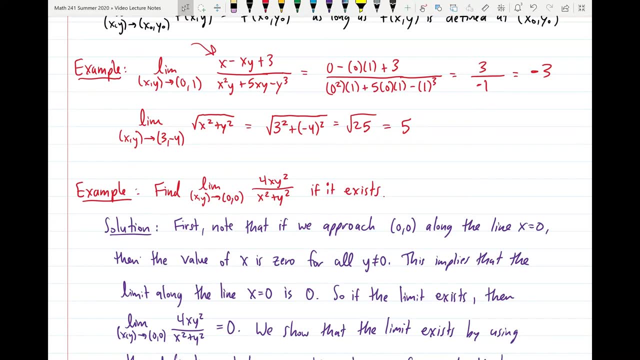 x and y respectively and we end up getting the square root of twenty five, which is equal to five. So because the function is defined when we plug in three negative four, then the limit, as x, y goes to three negative four of our function, is going to be equal to five, The value we get when we plug in 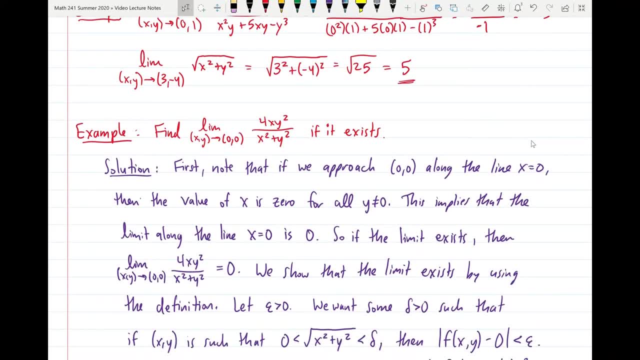 three negative four to the function. Okay, so now that we have those examples behind us, we are going to move into some examples that are significantly more difficult, And I know that they're significantly more difficult, so I understand that If you have trouble following along here, I think that's completely normal. Also, know that I don't 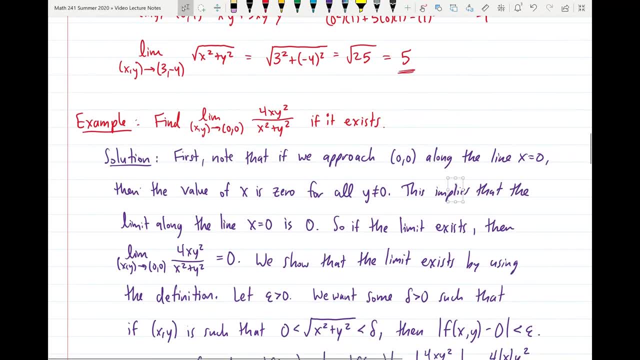 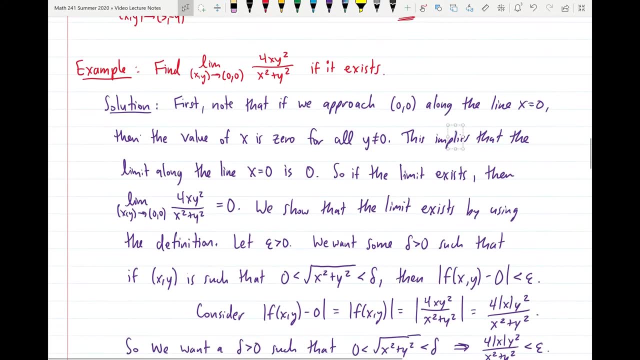 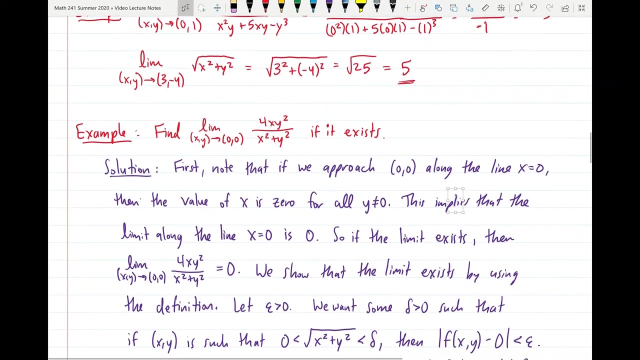 think I'm going to end up being super strict with these kind of proofs showing that a limit exists or does not exist, or showing that a limit is some value or not some other value. But I do want to see that you are attempting these kind of problems and I can tell you that I'm going to give you a. 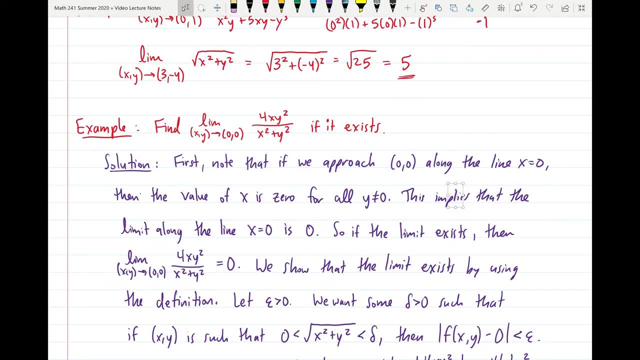 problem at least, where you have to plug in three negative four. So I'm going to show you that, I'm going to prove that the limit doesn't exist at some point for some function, And we'll get to some methods below that you can use to show that limits don't exist. But you can at least count on me. 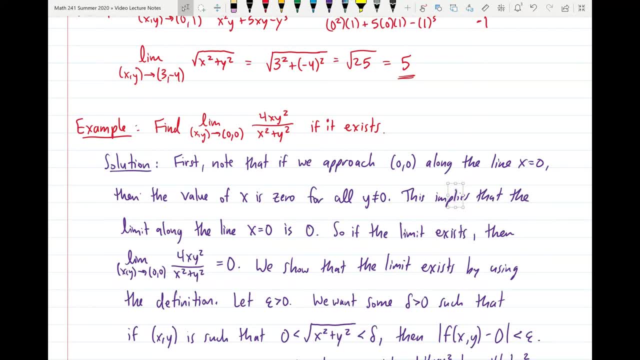 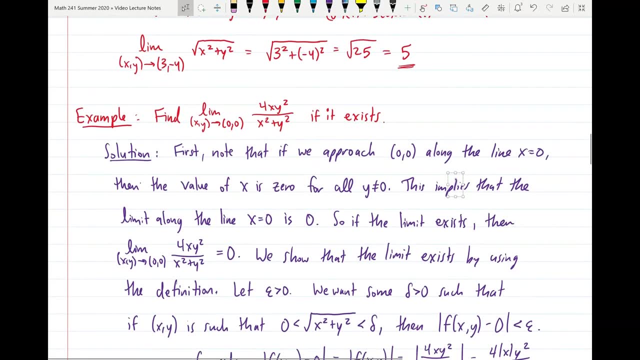 asking you at least one question where you have to show that a limit doesn't exist at a certain point. But in this example, we're going to show that a limit does exist. We're going to find what that limit is. So we're going to find the limit as x, y goes to zero, zero. 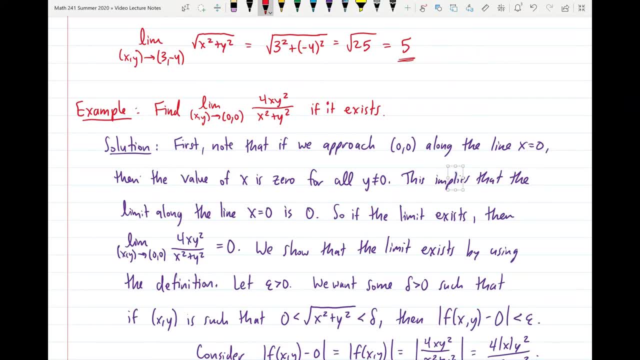 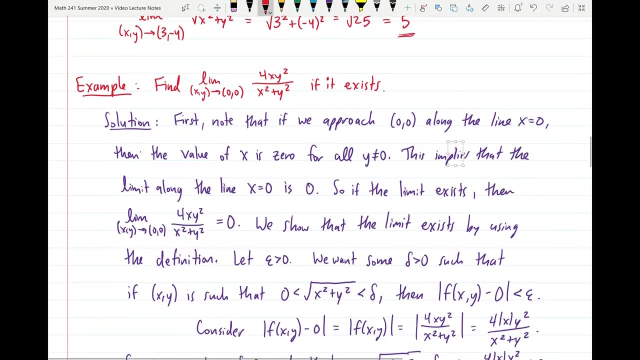 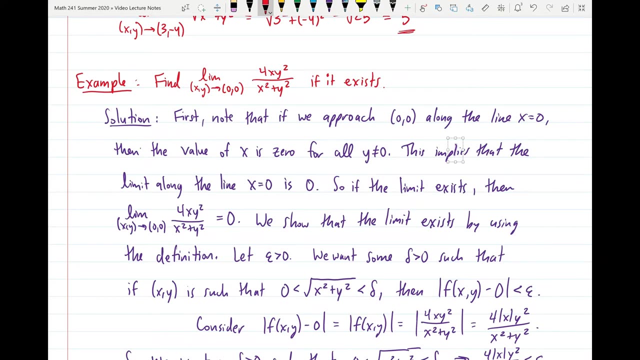 So we're going to find x, y squared divided by x squared plus y squared, if it exists. And spoiler alert, the limit does exist, which we will show below. So first we want to note that if we approach the value zero- zero along the line x equals zero, then the value of x is zero for all, y not equal to. 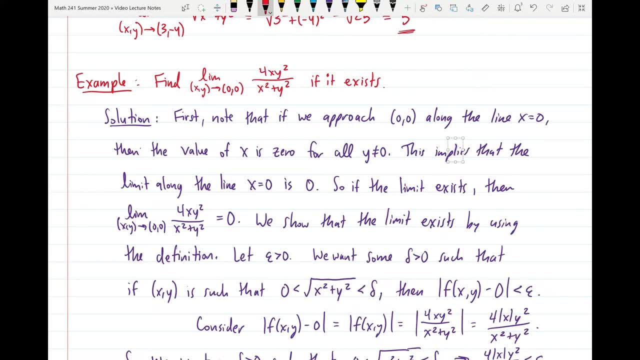 zero. So, first off, what do I mean by approaching the point zero? zero along the line x equals zero. Well, if you think about all of the points in the plane and then you think about the origin inside of the plane, Remember that as we take the limit, we're taking points and we are going. 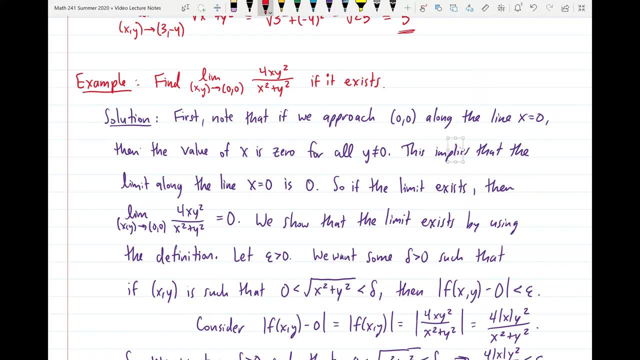 to be approaching the limit point Which, in this case, is the origin. But we can approach that limit point, the origin, from all kinds of different directions. Maybe we can approach it along the y-axis or along the x-axis, Or maybe we can approach it along the Y-axis or along the y-axis. 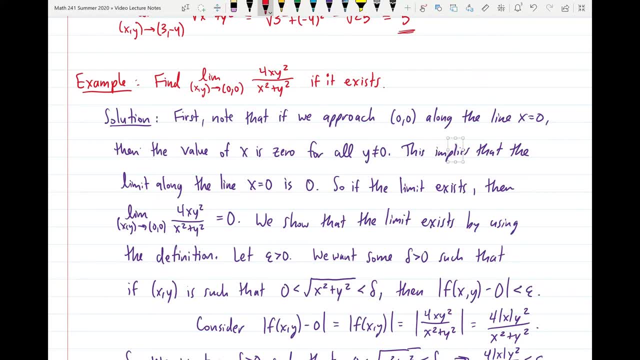 axis, or maybe we can approach it along a different line, or even a parabola. We have all kinds of different options in terms of what direction we are going to approach the origin from, And when I say along the line x equals zero, it means that we are going to approach it along the y-axis. 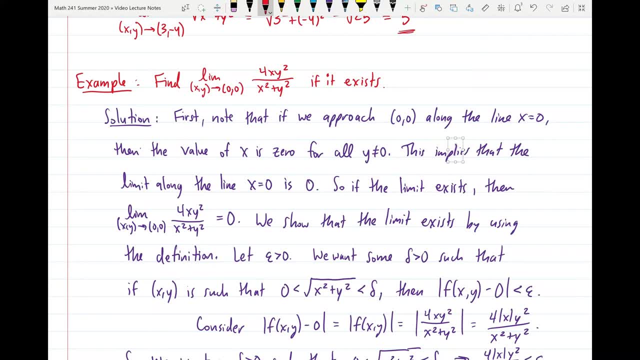 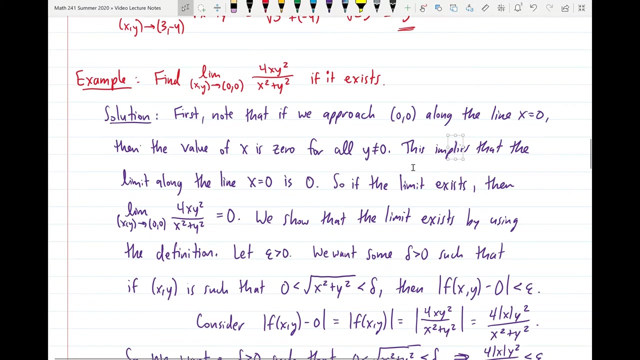 So we're going to get closer and closer to the origin as we're moving down the y-axis or up the y-axis towards the origin. So if we're approaching zero, zero along the line x equals zero, then the value of x is going to be zero for all of the points on that line And for that reason, if you 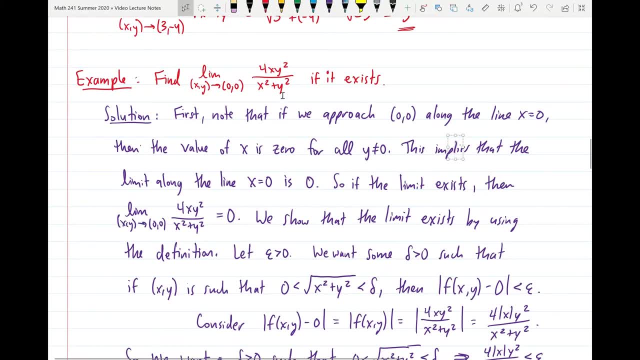 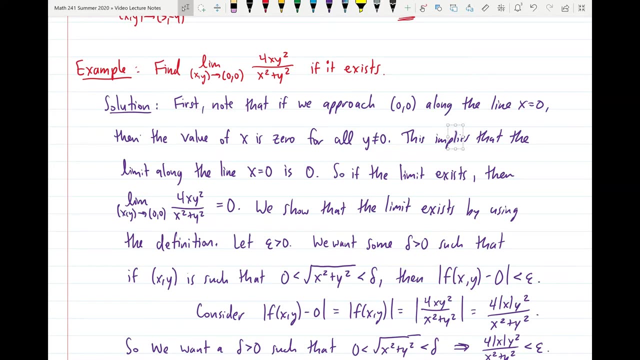 would take x equals zero and plug it into our function up here. you find that you get zero over y squared. And because we are approaching the point zero, zero, we're assuming that y is not equal to zero, in which case the function along the line x equals. 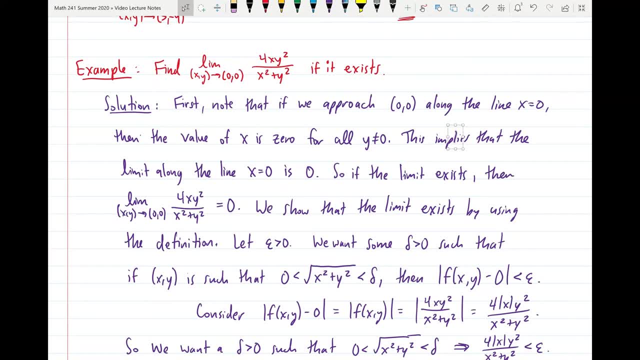 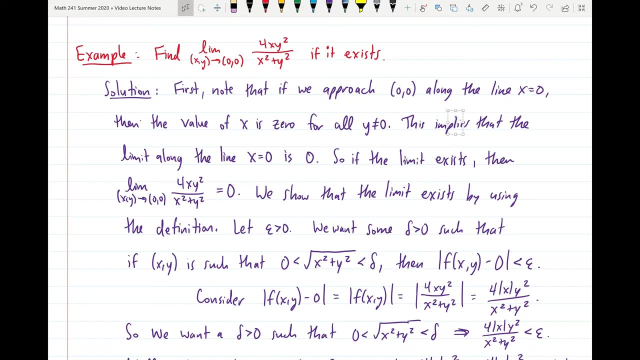 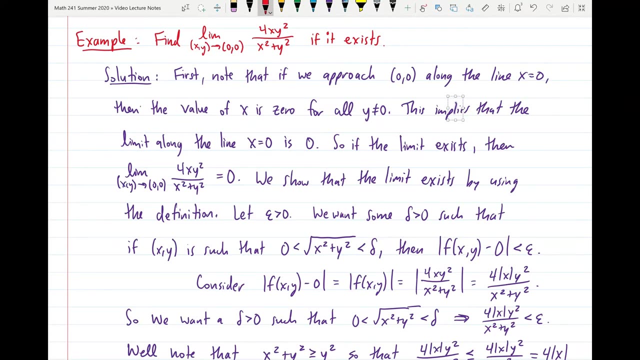 zero. where y is not equal to zero is going to equal zero. So the function is going to equal zero along the line x equals zero, as long as y does not also equal zero. But what this means is that limit, if it exists along the line x equals zero, is going to equal zero. And so if the limit exists, 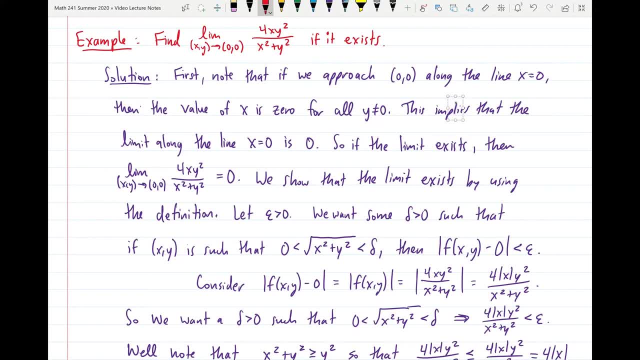 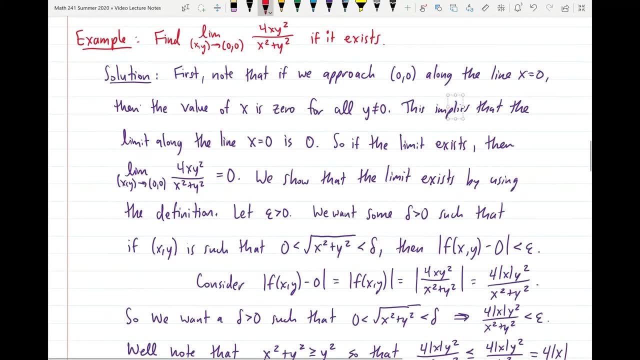 at all, then the limit has to equal zero. So this refers to something I don't think I've said yet. but if you have a limit of a multivariable function- and the limit does exist- then if you approach the limit point from all possible different paths inside of the plane, then you 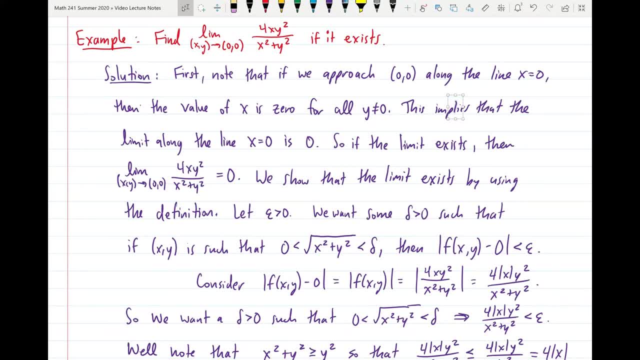 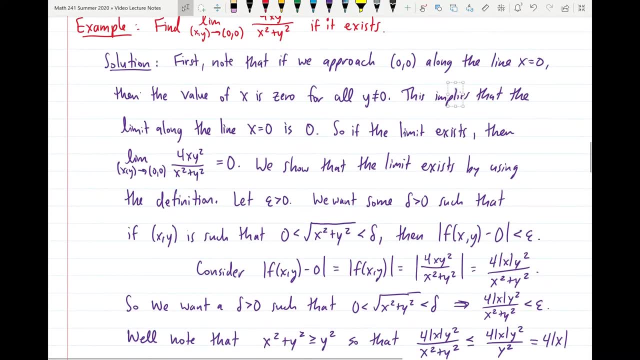 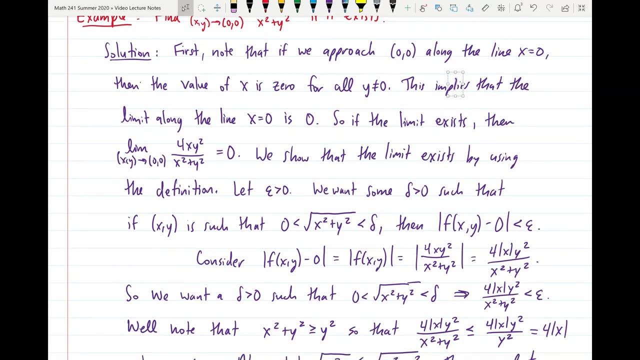 have to get the same limit, regardless of the path that you approach the limit point from. So, because we got, the limit is equal to zero when we approached along the line, x equals zero. it means that if the limit exists, then the limit has to equal zero. 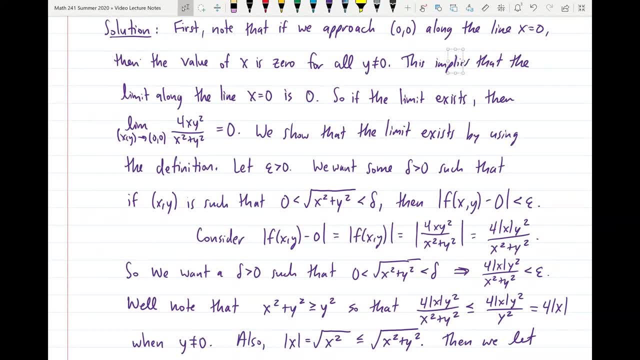 It doesn't necessarily mean that the limit exists. For example, I could approach along the line y equals zero and we could find that the limit along y equals zero gives us a different value, And if that was the case then the limit would not exist. But we know that if the limit does exist, then the limit has to equal zero. 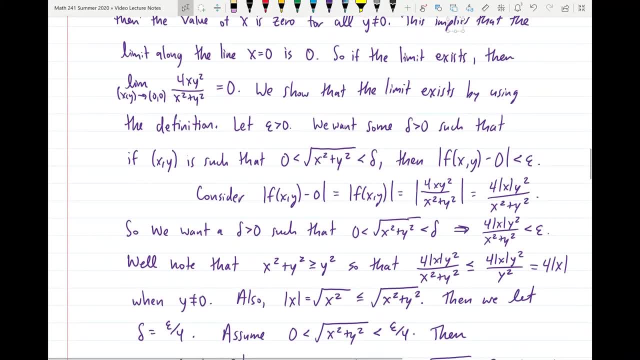 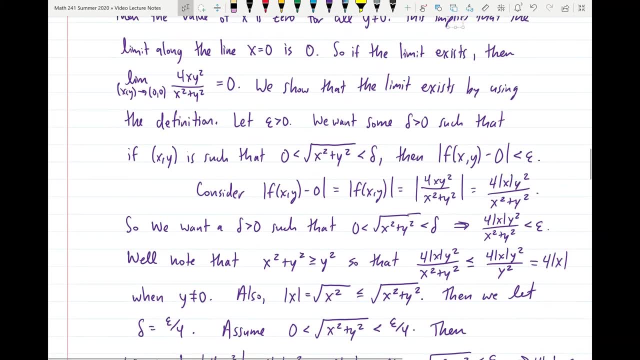 So now we have to show that the limit actually exists, because we know that if it exists, then it has to equal zero, And the only way we can do that is by using the definition of the limit. So this is where the example is going to get. 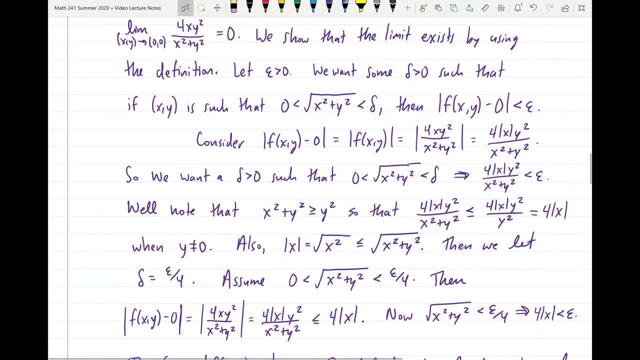 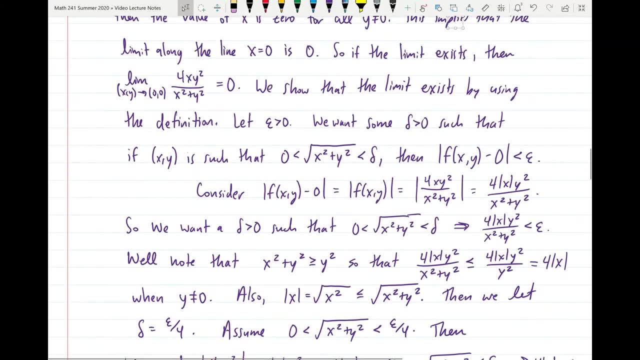 pretty difficult if you haven't seen this idea before, which I'm assuming you haven't, or maybe you've touched on it a little bit in Calc 1 or Calc 2.. But to do so we're going to use the definition of the limit, And so we let epsilon be some number greater than 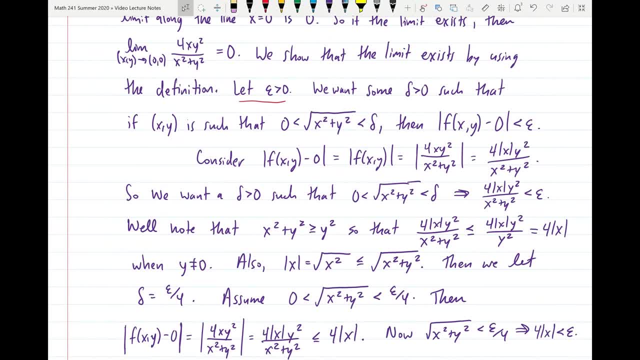 zero And to show the limit exists, we want to find some delta greater than zero, such that if the point xy is such that the square root of x squared plus y squared is between zero and delta, then it implies that the absolute value of f of xy minus zero is less than epsilon, Because- remember, 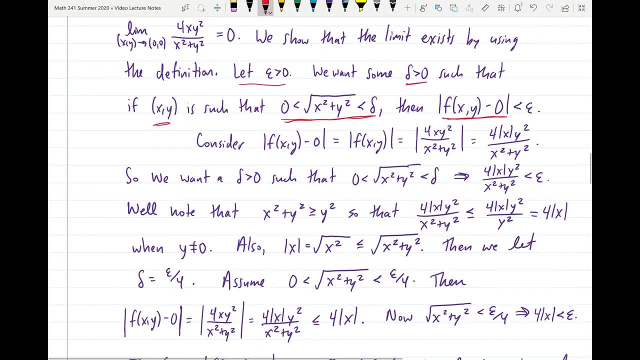 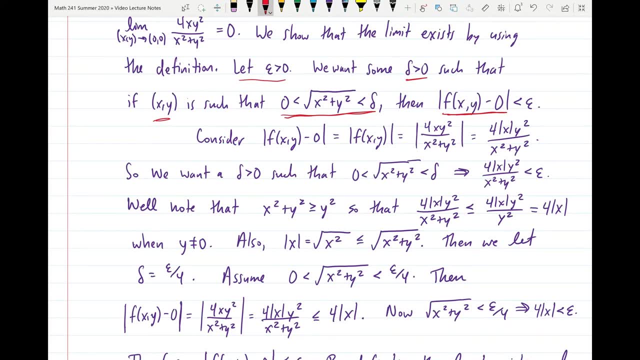 zero is going to be the limit point, if this limit exists. So now the absolute value of f of xy minus zero is of course the same as the absolute value of y, And then we can plug in the function for f of xy, So that's 4xy squared divided by x squared plus y. 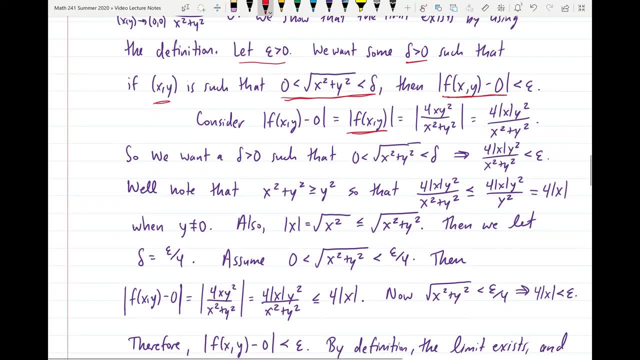 squared, We're still taking the absolute value of that, And now we can make that look a little bit nicer Because, remember, x squared plus y squared is always going to be greater than or equal to zero. So the absolute value of x squared plus y squared is just equal to x squared plus y squared. 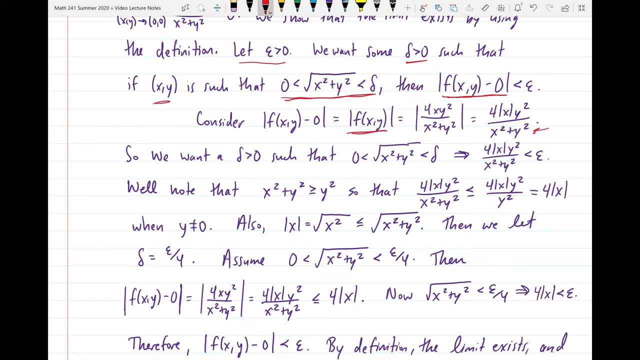 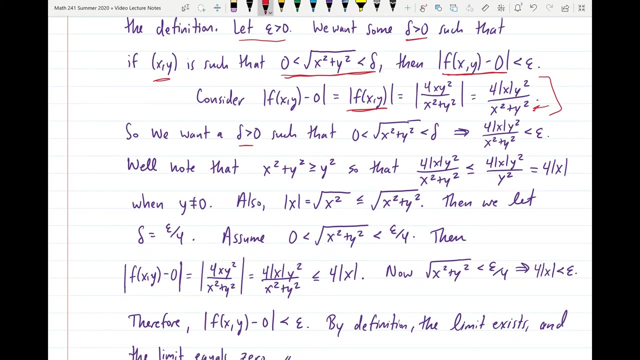 y squared is always going to be greater than or equal to zero, And four is of course greater than zero. So we can actually simplify it to this expression here, where we just keep the absolute value around the x, And so we want a delta greater than zero, such that if x squared 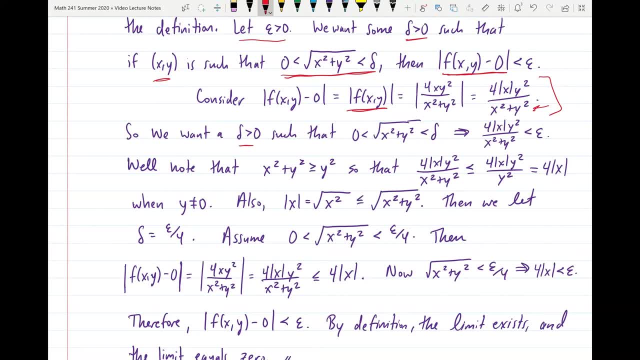 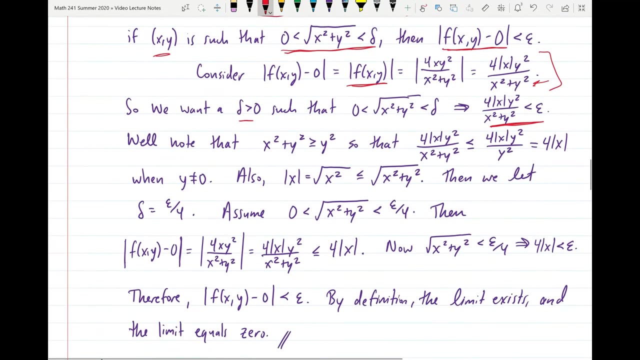 if the square root of x squared plus y squared is between zero and delta, then 4 times the absolute value of x times y squared over x squared plus y squared is less than epsilon. Again, this is just the definition of the limit here. Well, we can note that x squared plus y squared 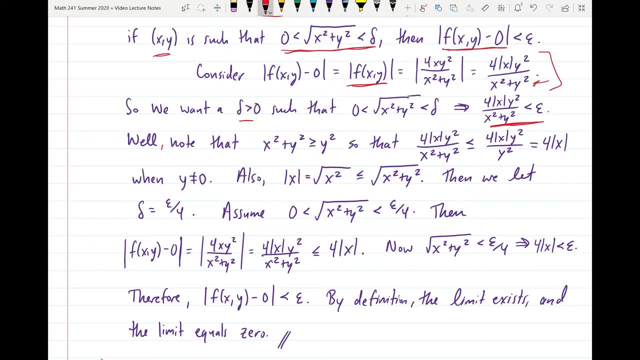 is going to be greater than or equal to y squared, regardless of what x squared or y squared we choose, because x squared and y squared are both greater than or equal to zero, And so this implies that 4 times the absolute value of x times y squared over x squared plus y squared is less. 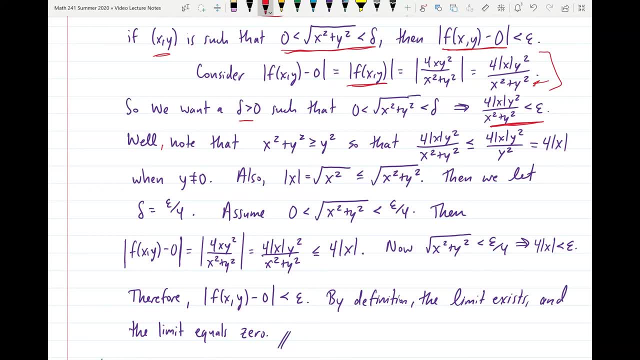 than or equal to 4 times the absolute value of x times y squared over x squared plus y squared, Because, remember, x squared plus y squared is greater than or equal to y squared, implying that this guy has to be less than this guy. And now, as long as y is not equal to zero, 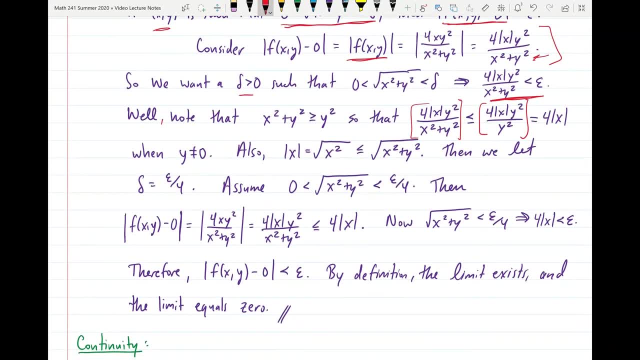 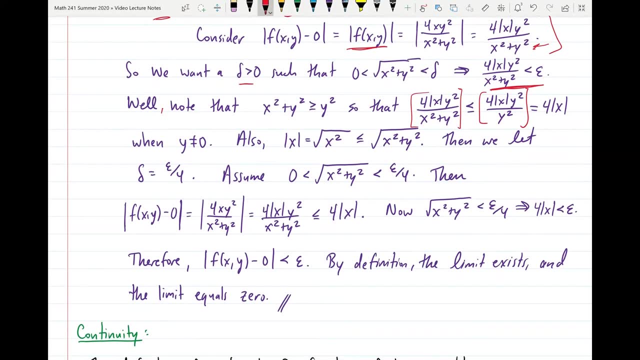 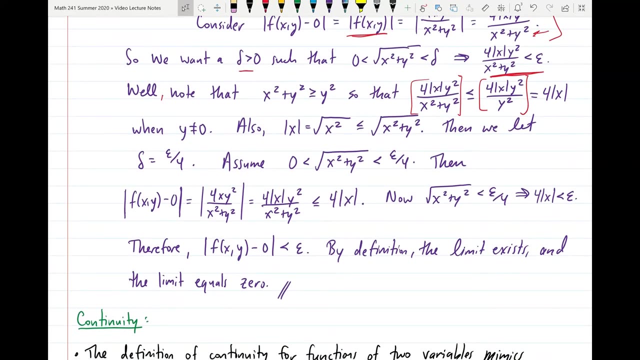 and this expression is equal to 4 times the absolute value of x. And that's okay, because we're assuming that y doesn't equal zero, because the limit point is zero, zero. So we're going to calculate the absolute value of x times the absolute value of y squared over x squared. 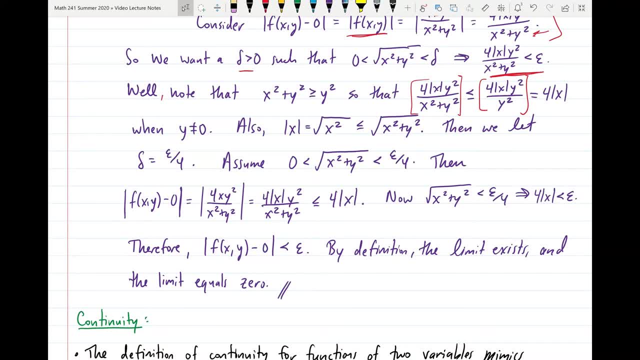 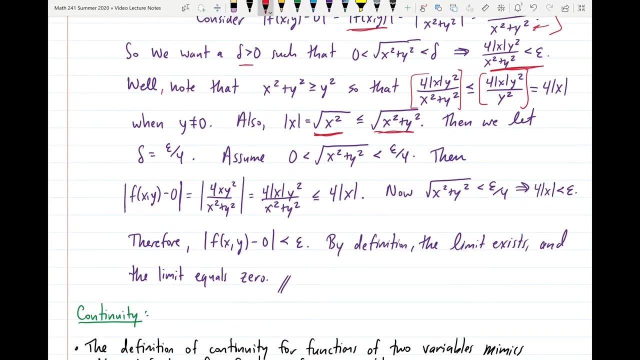 Also, the absolute value of x is equal to the square root of x squared, and that's going to be less than or equal to the square root of x squared plus y squared for all y, Because, again, y squared is always going to be positive, or greater than or equal to zero. I should say: 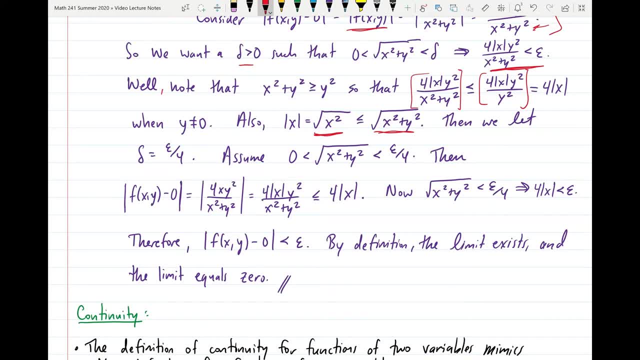 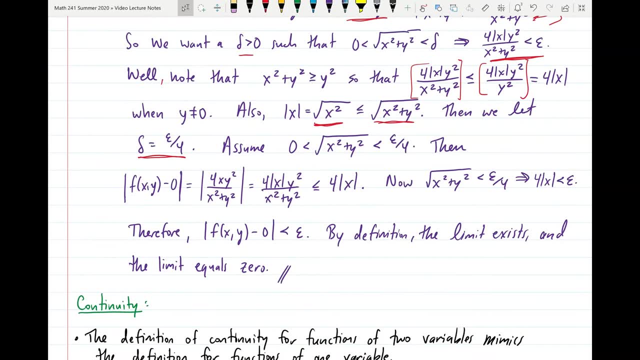 And for all of these reasons, we're going to let delta equal epsilon over 4.. And I think the reason we let delta equal epsilon over 4 is going to become clear once we go through these next couple of steps. So assume that we have some point: x y And x? y is such that the square 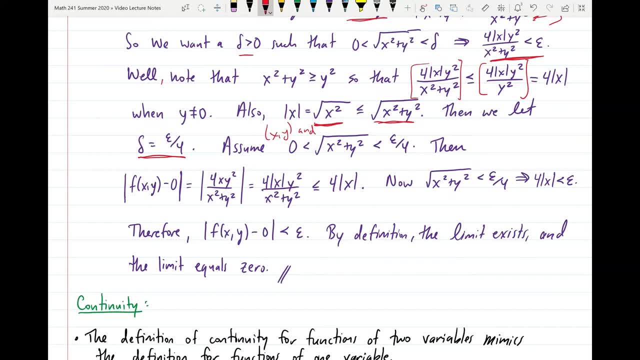 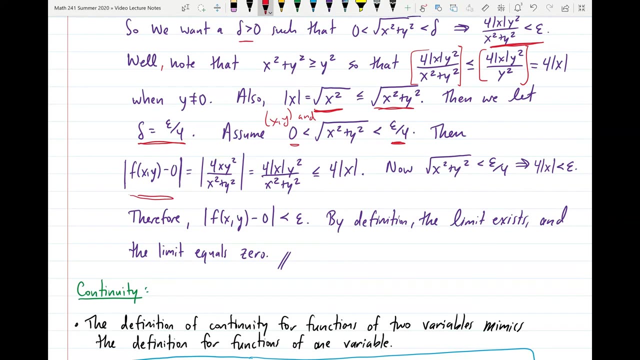 root of x squared plus y squared is between zero and epsilon over 4.. Here we've let delta equal epsilon over 4, and we need to show that f, that the absolute value of f of x, y minus zero is less than epsilon. That's our ultimate. 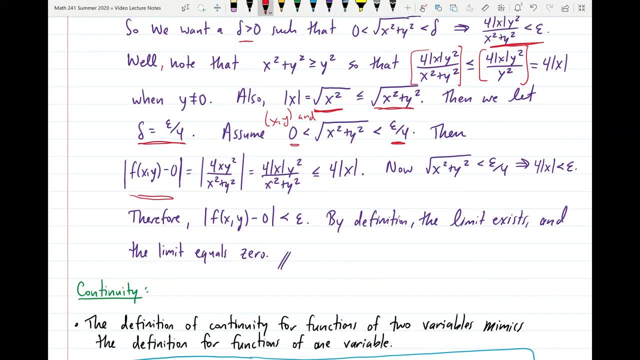 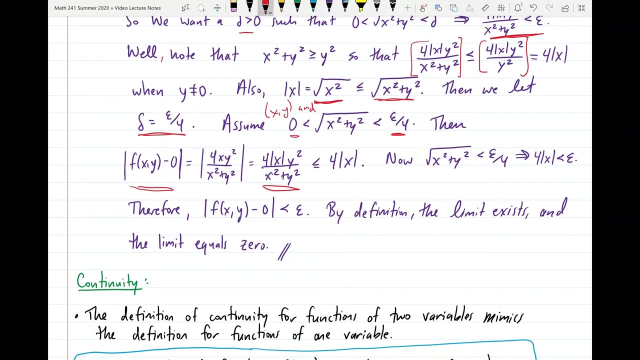 goal here. Then we can write: the absolute value of f of x, y minus zero is equal to, ultimately, this: four times the absolute value of x times y squared, divided by x squared plus y squared, and we already said that that's going to be less than or equal to four times the absolute value of. 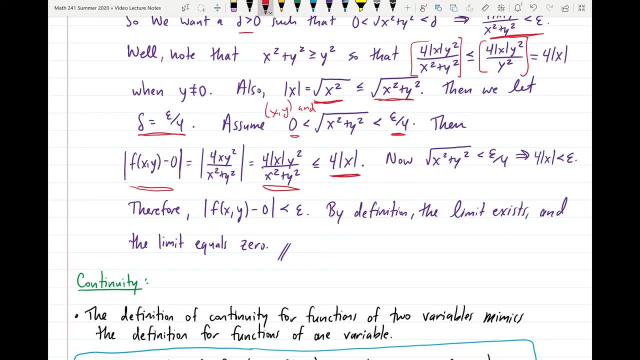 x and we also said that because the absolute or because the square root of x squared plus y squared is less than epsilon over four, and because we already said up here that the absolute value of x is less than or equal to the square root of x squared plus y squared, which is less than epsilon, 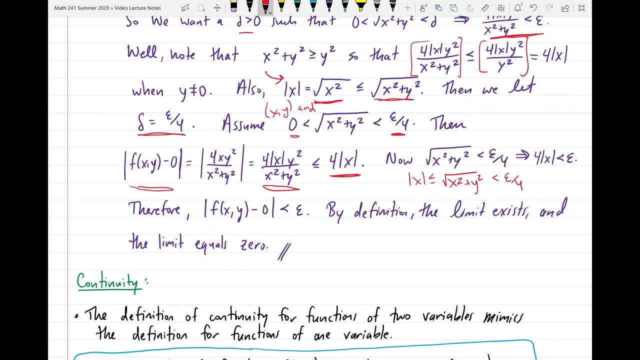 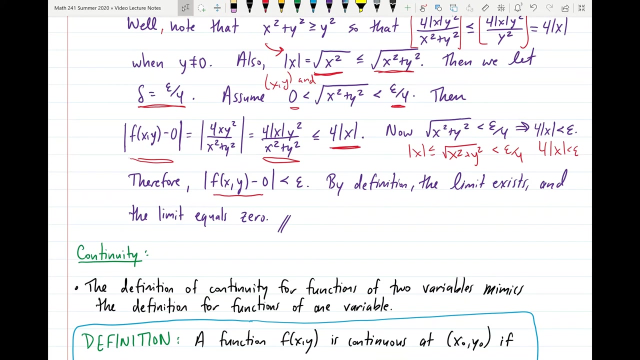 over four, We can use this inequality to say that four times the absolute value of x is less than epsilon, and so this ultimately means, then, that the absolute value of f, of x, y minus zero is less than epsilon. So we picked a delta which happened to be epsilon over four, such that if the distance 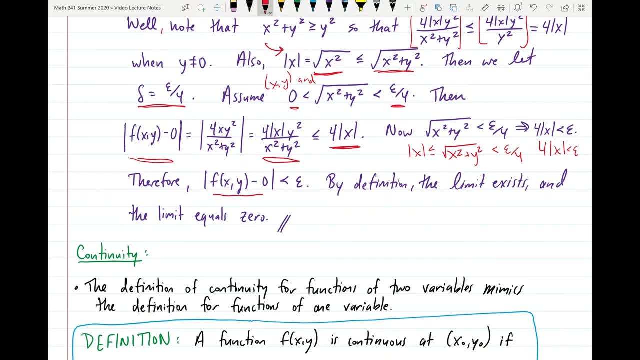 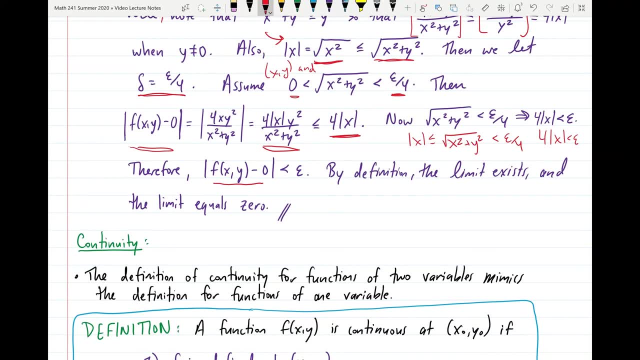 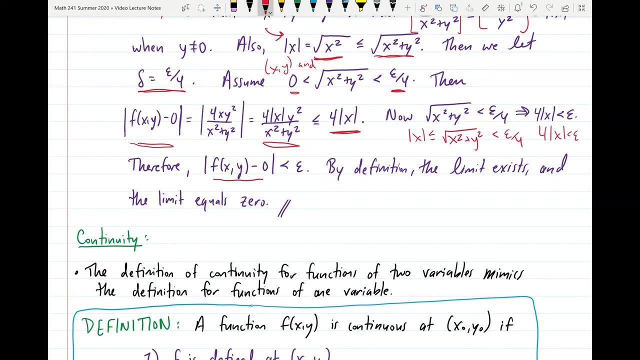 from our point to the origin is between zero and epsilon over four, then the distance from f of x, y to zero is less than epsilon and for this reason, by definition the limit exists and the limit is equal to zero. So I am completely aware that for the majority of 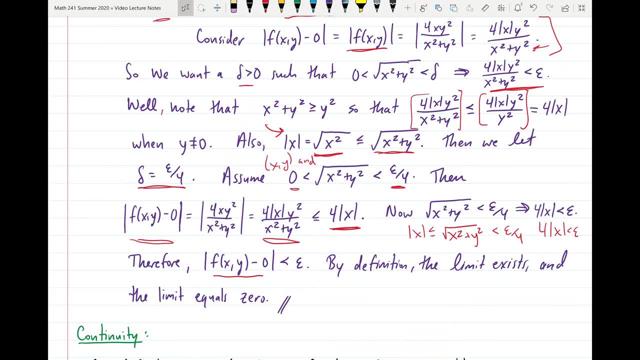 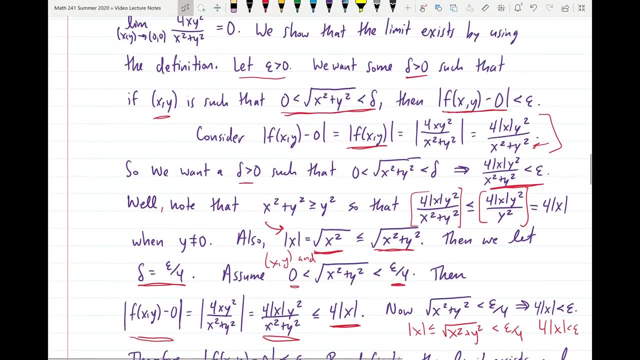 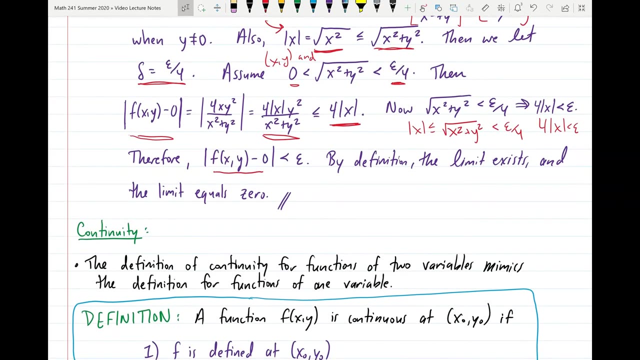 people. this proof that I just gave to say that the limit is equal to zero is super foreign and probably difficult to follow, and that is okay. I would actually just encourage you to go on to blackboard and find my lecture notes and read through this proof. a couple of different. 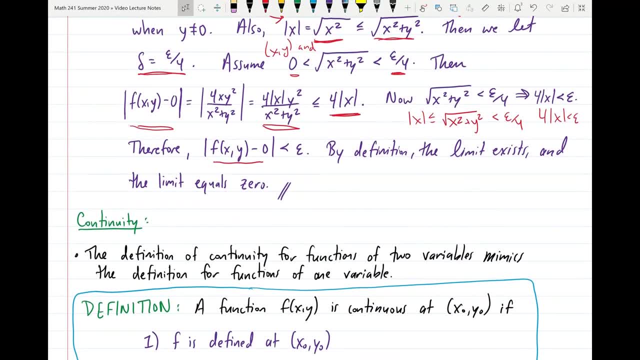 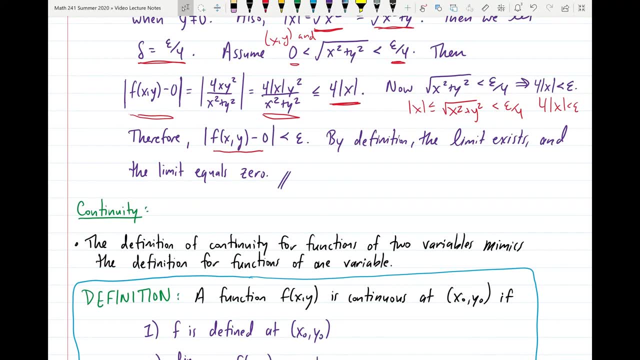 times until you feel comfortable, like you understand generally what's going on inside of the proof. So the idea is we pick some epsilon greater than zero and we need to find a delta greater than zero such that the conditions for the definition of a limit are met. That's the. 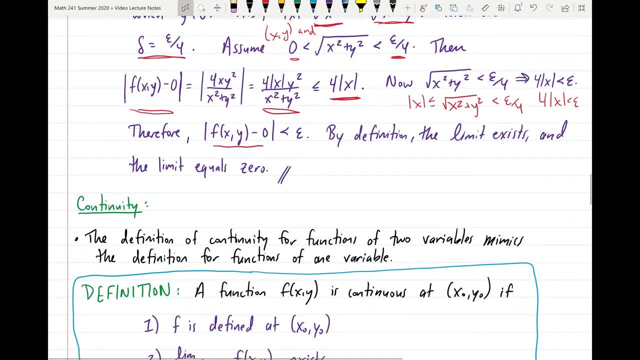 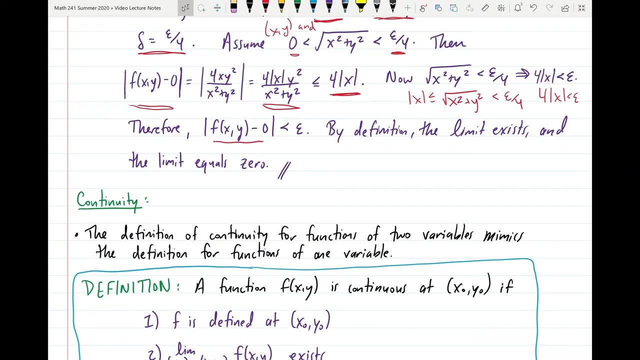 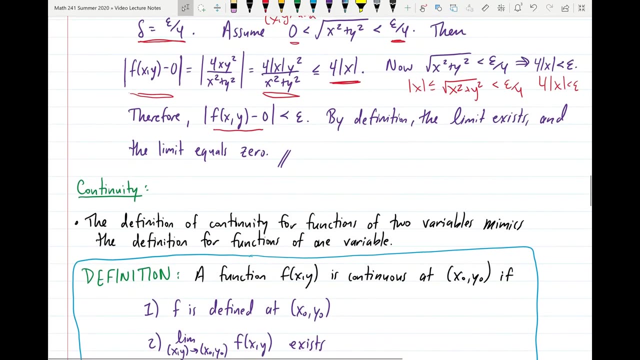 general idea and then the question is: what are the little nitpicky things that we have to do to make sure that that we can actually find that delta? So read through the proof that I have multiple times and also email me questions about the proof or things that you don't understand, if you find. 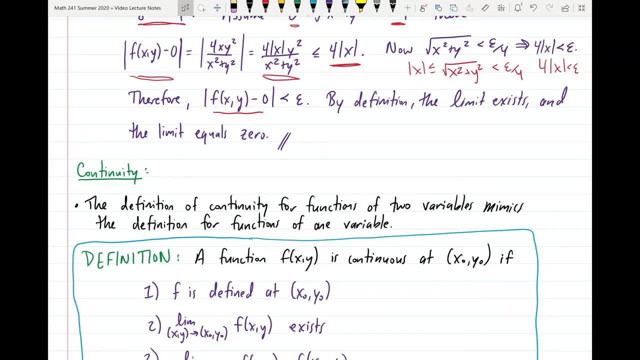 that you're really struggling to understand it. I am going to give probably at least one homework problem where you're going to be evaluating or proving that a that a limit exists for a function that is equal to zero. So I'm going to give probably at least one homework problem. 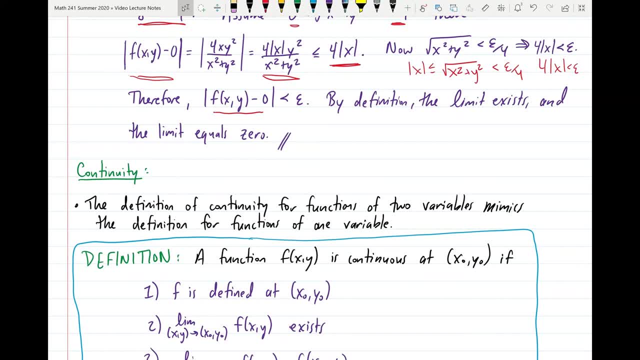 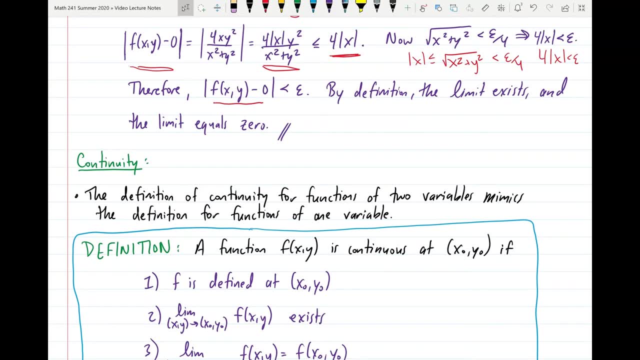 where you're going to be evaluating or proving that a that a limit exists for a function like this. So you're going to get a little bit of practice, but not too much. So so email me if you have any questions or there's confusion related to the proof that I just gave. Okay, so now that 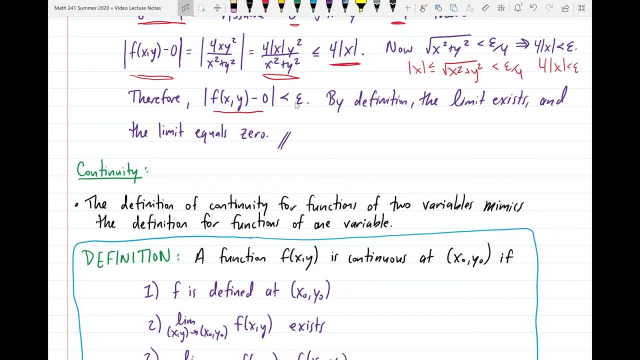 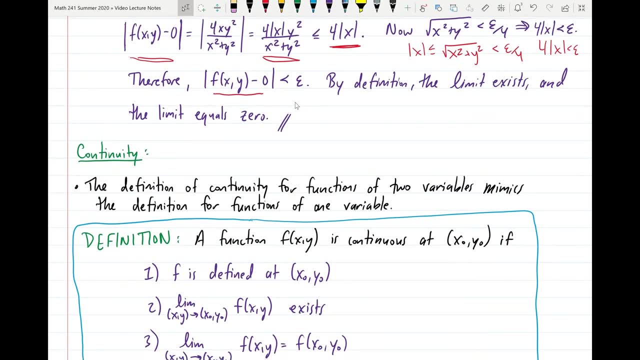 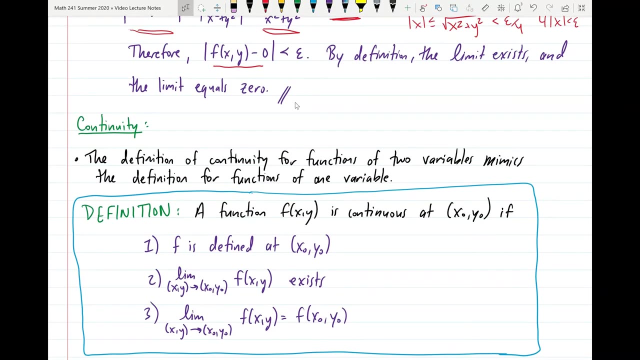 we've talked about limits for multivariable functions, it makes perfect sense to move on to the idea of continuity, which is exactly what we moved on to with vector valued functions, and it's what we moved on to when we introduced limits for for single valued functions back in calc one. So the definition of continuity for functions of 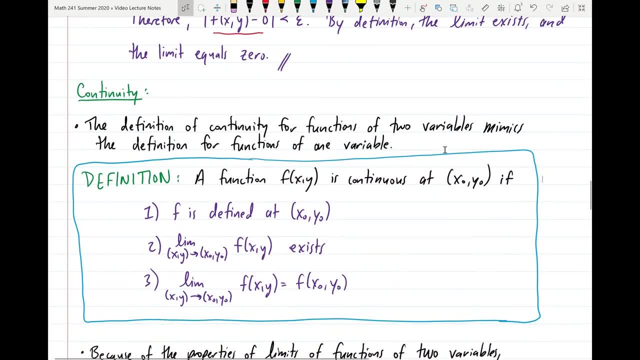 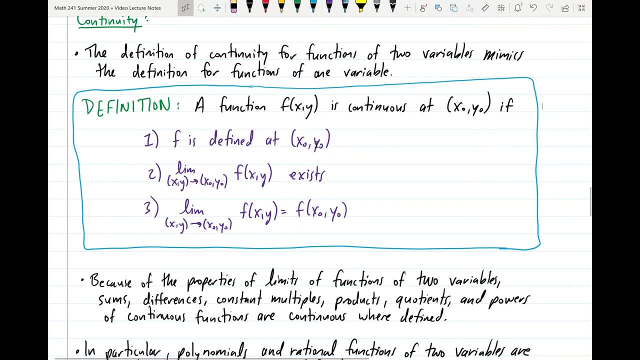 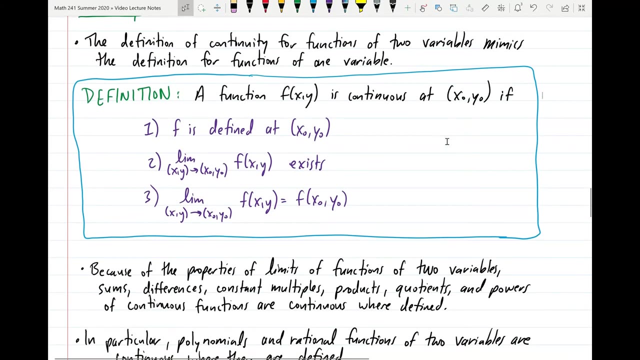 two variables and ultimately any multivariable function mimics the definition for functions of one variable, So I'll just give the definition here. it should be familiar. A function f of x- y is continuous at the point x naught, y naught if the following three conditions are satisfied: 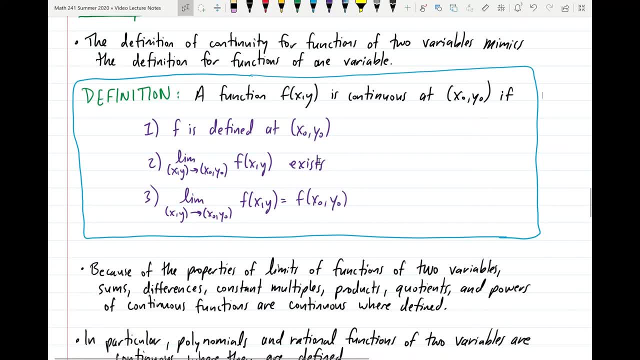 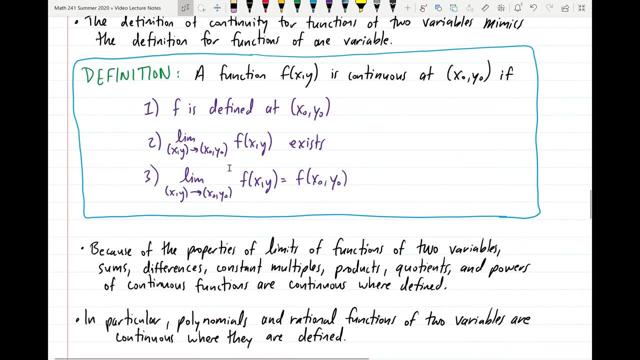 So one f has to be defined At the point x, naught y naught. it has to make sense to put the point x- naught y naught into our function. The second condition: the limit, as x- y goes to x naught, y naught of f of x- y. 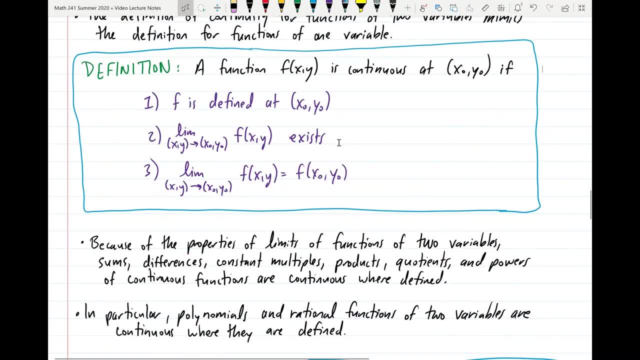 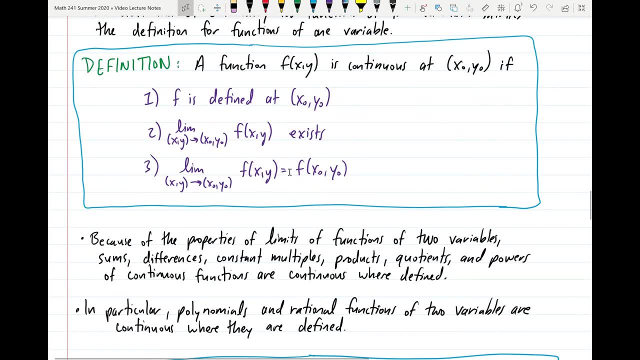 has to exist. That's the second condition. and then the third condition is that the limit, as x- y goes to x, naught y naught, of f of x, y is actually equal to f of x, naught y, naught, So the limit is going to equal the value. 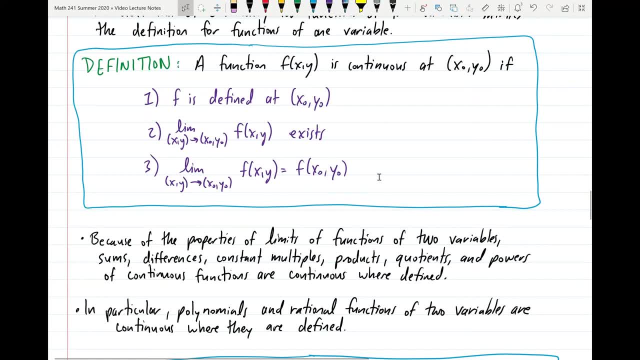 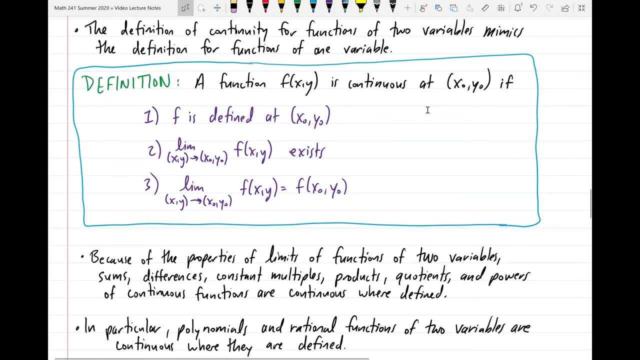 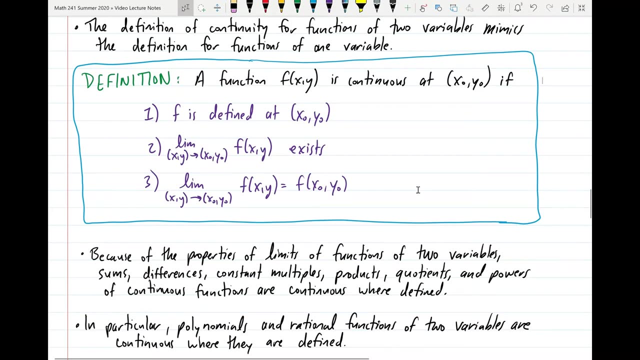 we get when we plug in the limit point to the function. So if all of these conditions are satisfied, we say that the function is continuous at the point x, naught, y, naught, And more than just that. we say that a function is continuous just generally if it's continuous at all of the points. 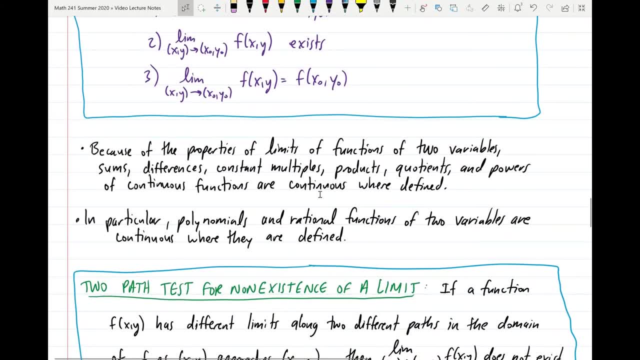 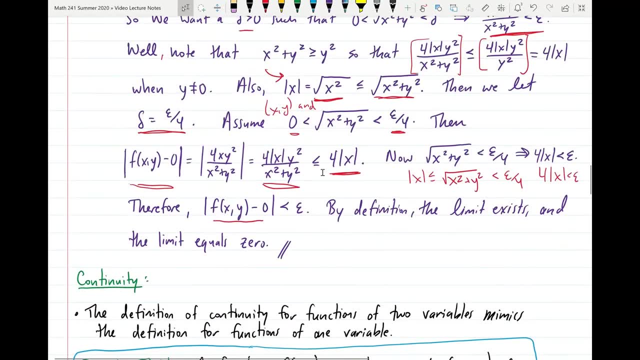 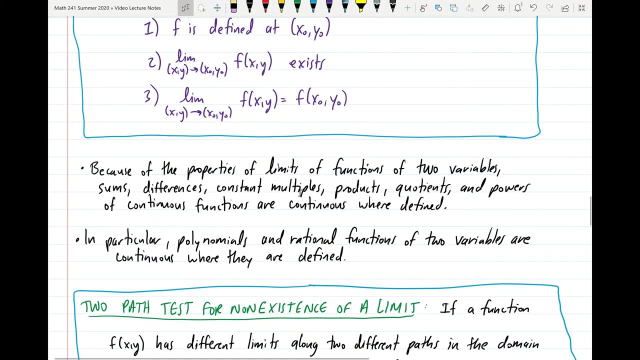 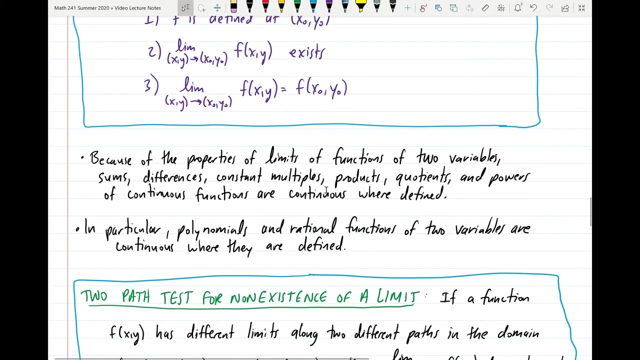 in its domain. So because of the properties of limits of functions of two variables. so the properties that I listed in this box up here, because those properties hold, we can say that sums, differences, constant multiples, products, quotients and powers of continuous functions. 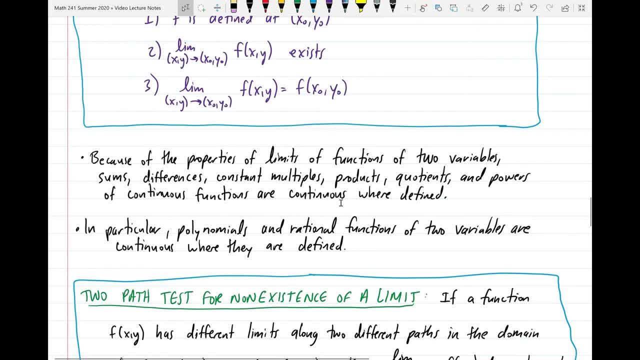 are also themselves continuous whenever they're defined. So what that means is that if I have a continuous function and another continuous function and I add them together, I get a continuous function. If I subtract them, I get a continuous function. If I multiply them by a constant, I get a continuous. 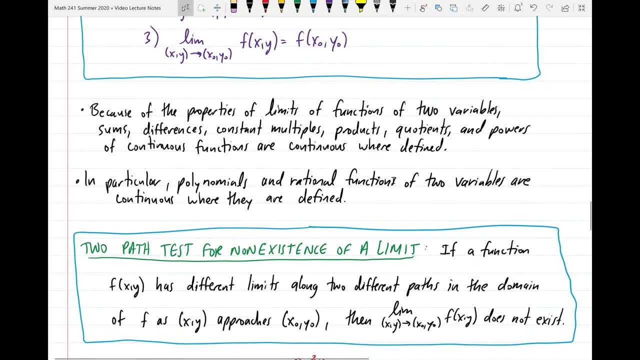 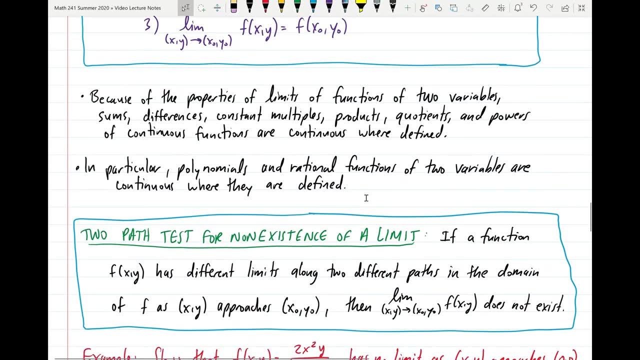 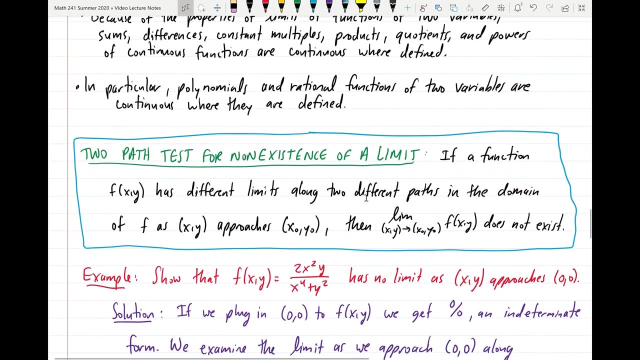 function and so on. for all of these properties here, And in particular polynomials and rational functions of two variables are continuous whenever they are defined. So that's an interesting thing to note. Make sure you remember that, because that's an easy way to just say right off the bat. 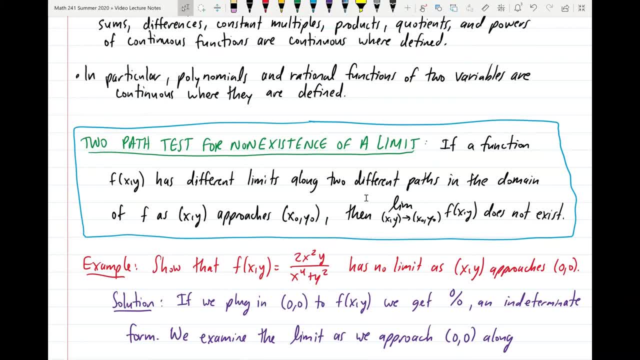 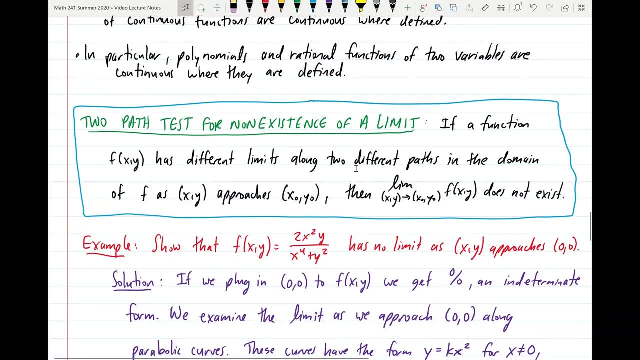 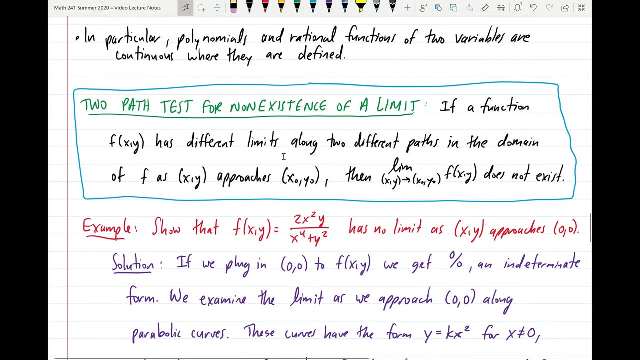 that a polynomial or rational function is continuous. Okay, and now let's move on to something that I alluded to before, when I gave that example of proving a function had a limit. We have what is called the two-path test for the non-existence of a limit. So this test is only 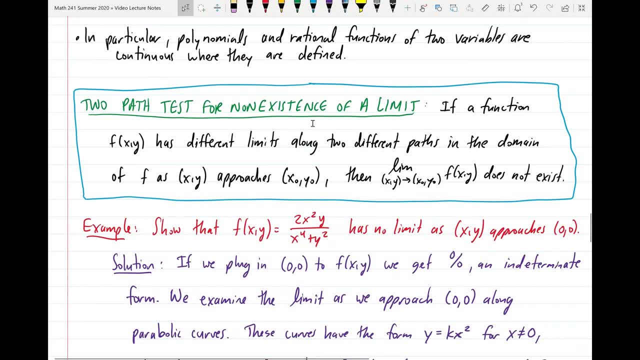 going to give us the non-existence of a limit. It is not sufficient to give us the existence of a limit. So the test says this: If I have a function f of x- y and if that function has different limits along two different paths in the domain of f, as x, y approaches x-naught, y-naught, then the limit 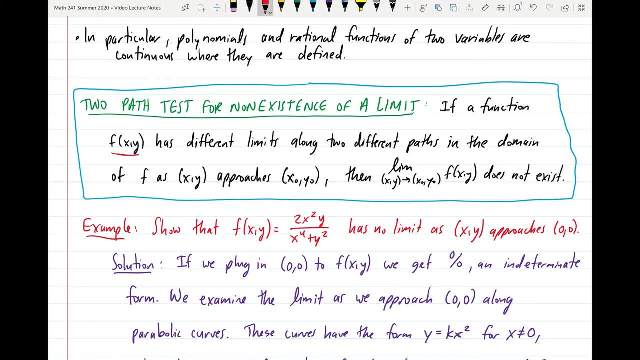 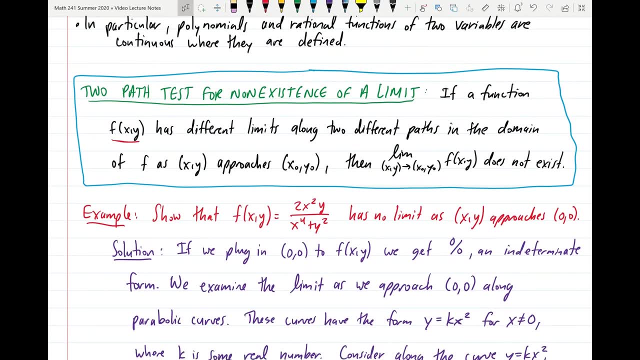 as x, y goes to x-naught, y-naught of our function does not exist. So let me say that again: If I have a function f of x, y and if that function has different limits along two different paths in the 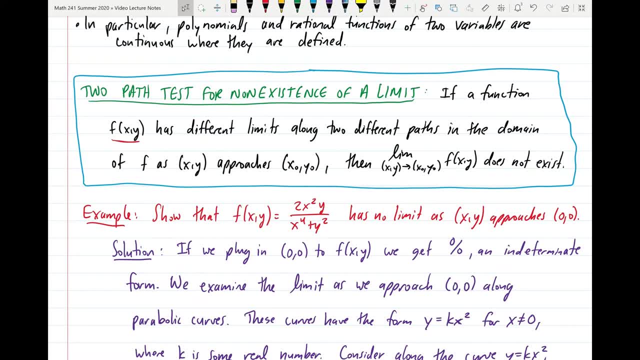 I approach a limit point from two different paths that are in the domain of my function and the limit that I get as I approach along different paths. if these limits do not equal one another, then the limit- as x, y goes to x naught, y, naught of my function, does not exist, so the limit. 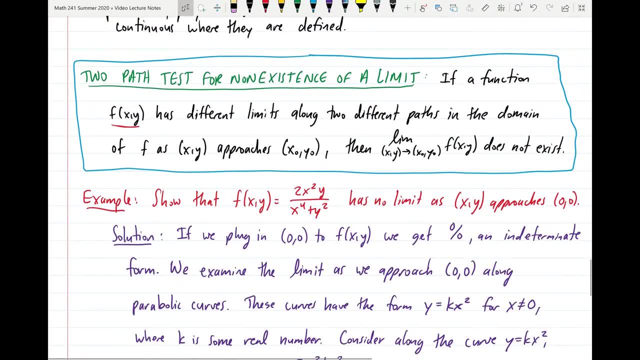 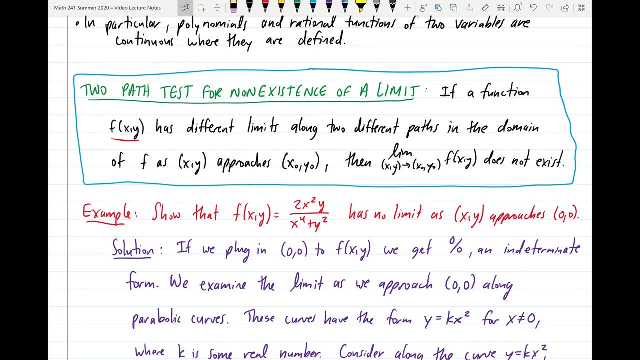 does not exist at that point. if this is the case- but again, this is not- this test is not sufficient to show that a limit does exist. so if I just pick two arbitrary paths and and I approach my limit point along these two different paths and I find that the limits along the two different paths are, 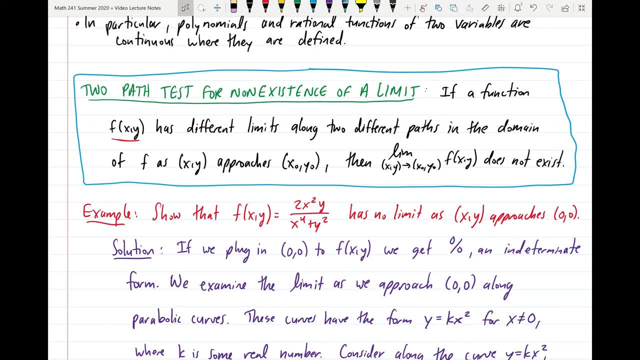 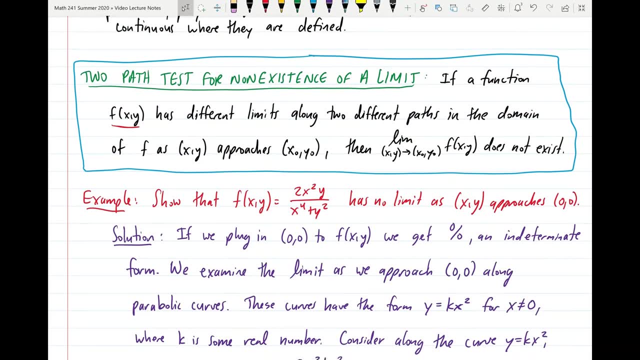 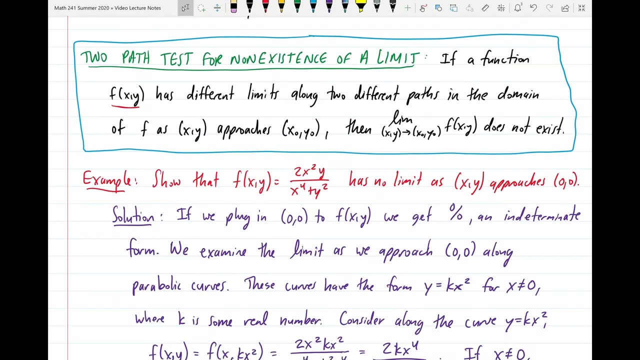 equal, it is still very possible that the limit will not exist. for that point, it's not sufficient to show that the limit exists along two different paths, to say that the limit, the limit, exists in general. to show that the limit exists in general, you really do have to go back to the 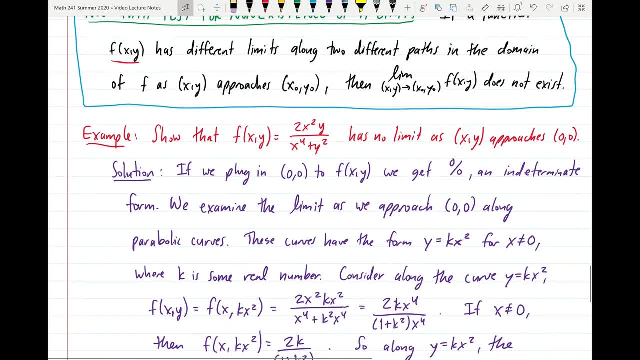 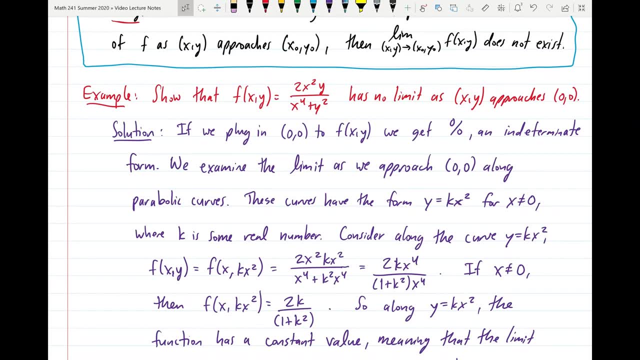 definition of the limit, just like I did in the example that I showed previously. so let's give an example where we are using this test. we want to show that the function f of x- y is equal to 2x squared times y divided by x to the fourth plus y squared, has no limit as x y approaches. 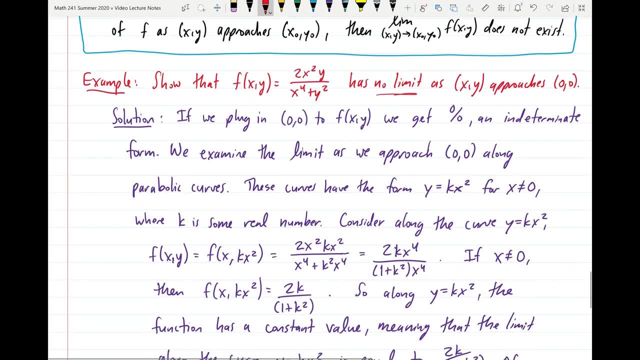 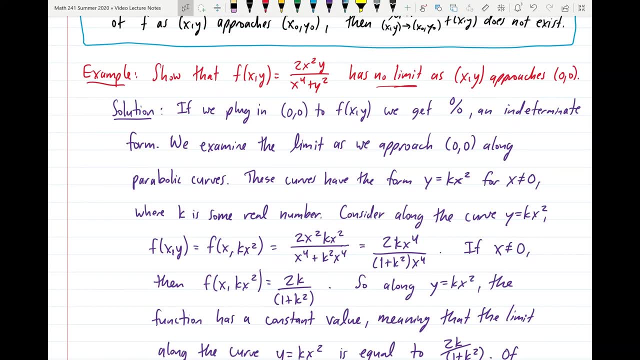 the origin or the point: zero, zero. so we want to find two different paths such that when we approach the origin along these two different paths, our function has different, has a different limit along the different paths. so let's start off by plugging in zero, zero to our function, because we should notice that our function is a rational. 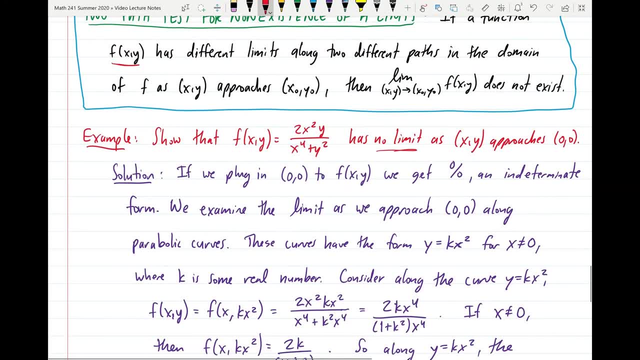 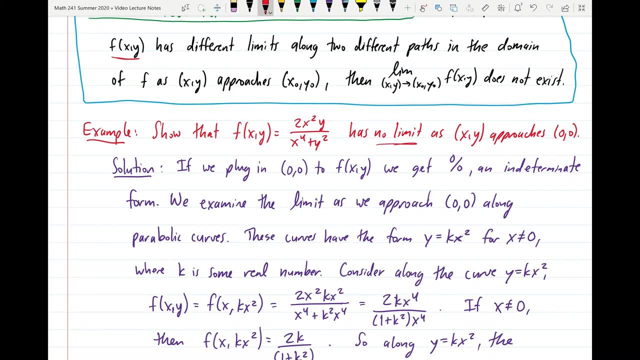 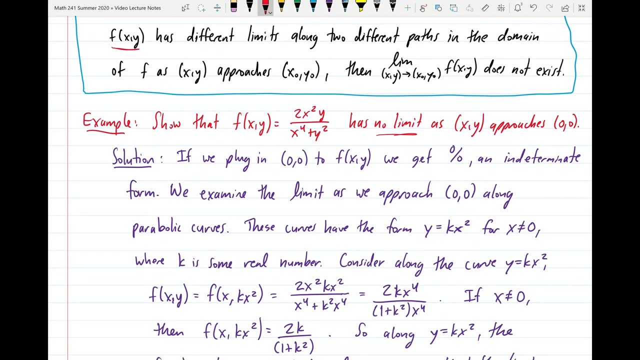 function, and for that reason if the function is defined at the point zero, zero, then the limit is going to exist. so we already talked about that property of rational functions before. but the problem is that if we take the point zero- zero and we plug it into our 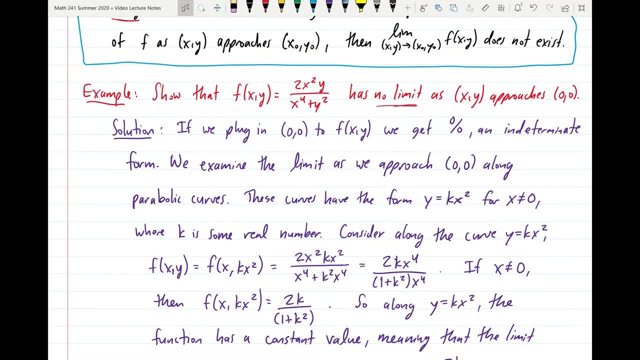 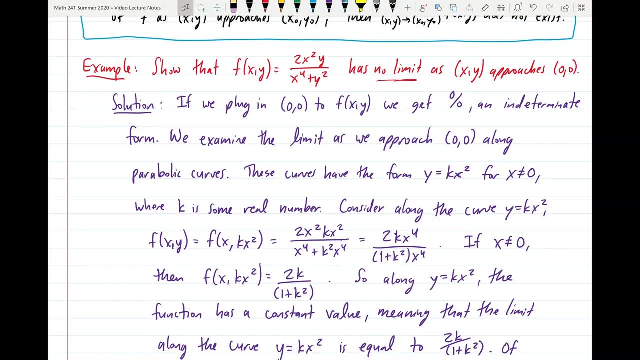 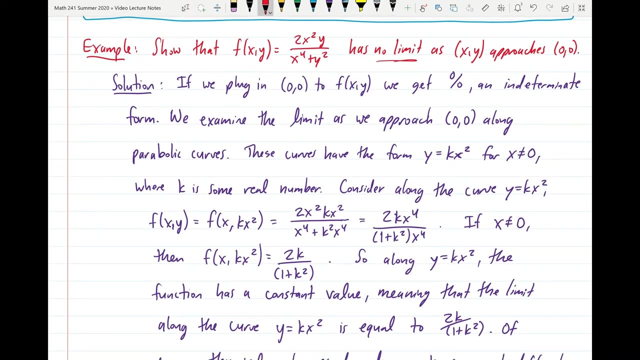 function f, we get zero over zero, which is an indeterminate form. so the function is not defined at zero zero. so we're going to have to do a little bit more investigation to see whether the limit exists or not. so we are actually going to examine the limit as we approach. 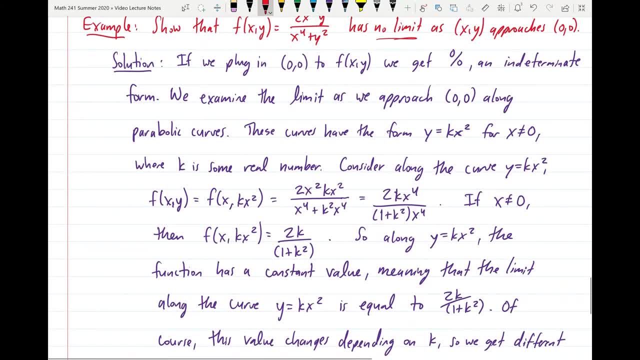 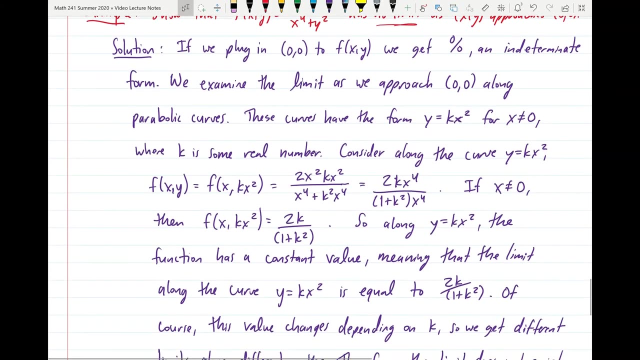 the origin along parabolic curves. so in the other example we approached the origin along the line x equals zero, and i talked about approaching the origin along the line y equals zero, so going down towards the origin. in this case we're going to talk about approaching the origin along parabolas. 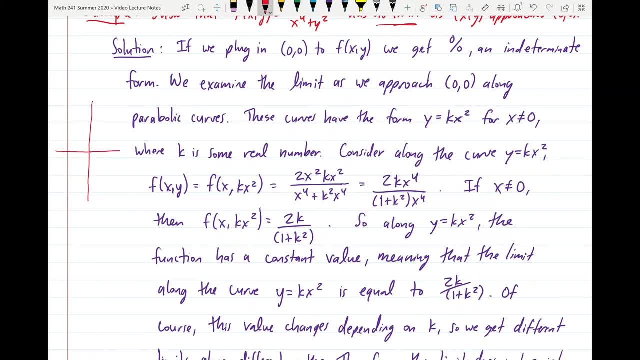 so if i draw a plane here and then the origin is going to be at the center of course, then we are going to have to do a little bit more investigation to see whether the limit exists or not. so if we draw a plane here and then the origin is going to be at the center of course, then we are going to 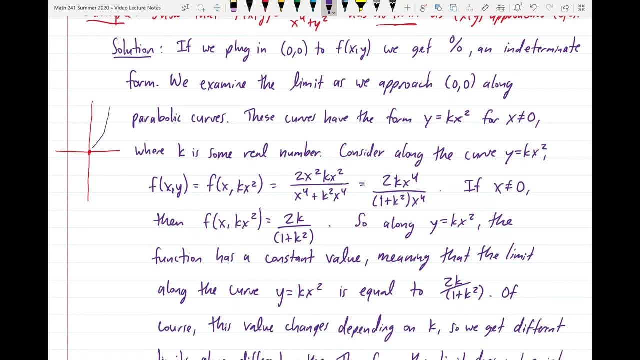 approach the origin along curves that look like this: down towards the origin. we can go down towards the origin from this direction. we can go towards the origin from this direction. the point is that all of the directions or the paths that i'm using to get to the origin are parabolas. 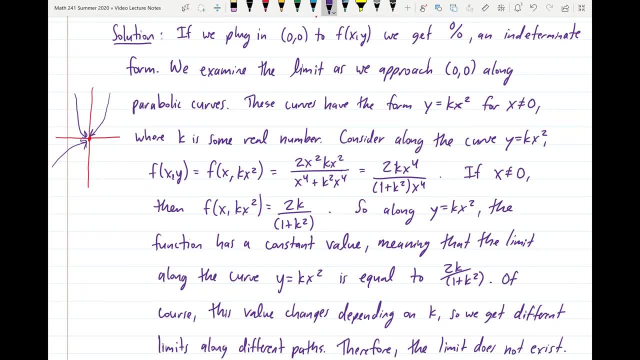 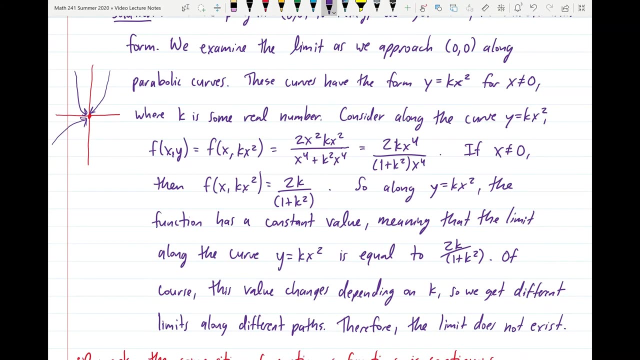 and so these curves have the form y equals k, x squared generally, where k is just some real number and we are not including the point x equals zero, because that's our limit point here. so consider along the curve: y equals k, x squared, where k is just some arbitrary real number. 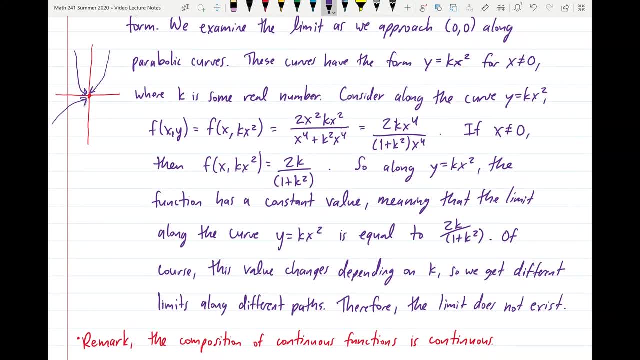 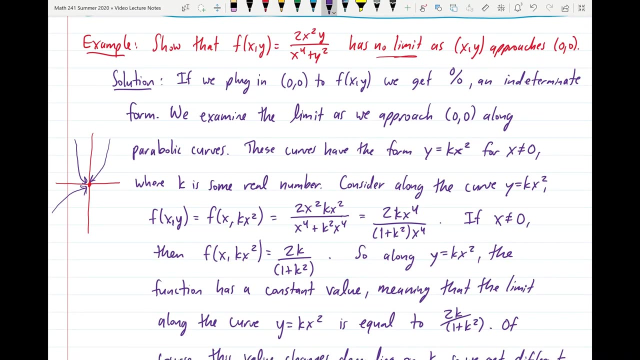 we have that f of x, y is equal to f of x, k x squared. so here we've taken k x squared and we've substituted it for y, and then, if we plug that into our function, we get 2 x squared times k x squared as our numerator, and then on the bottom we have x to. 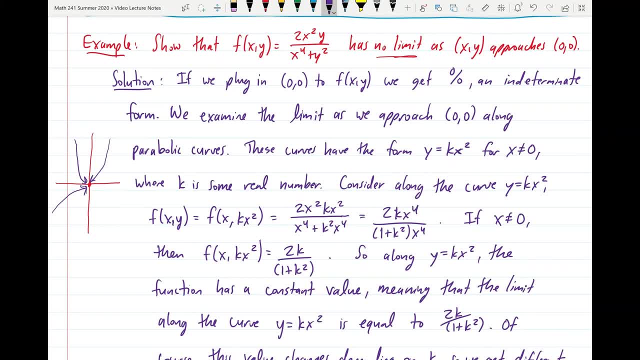 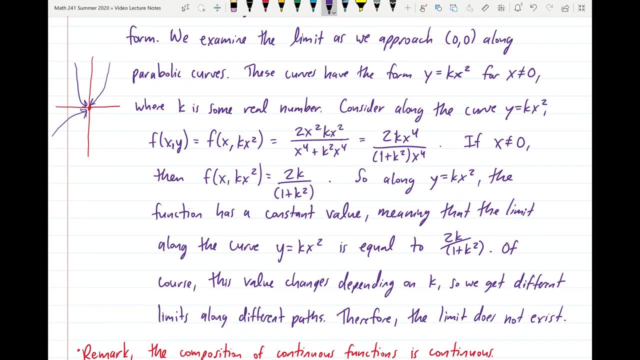 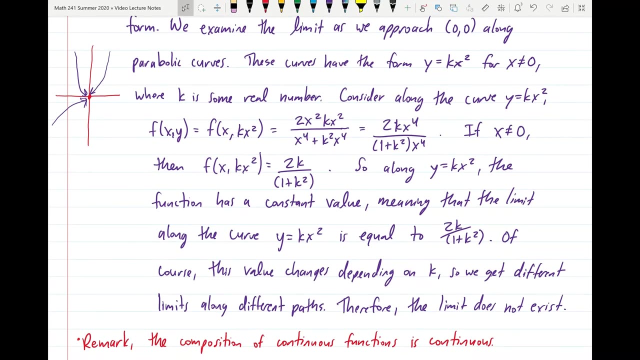 the fourth plus k squared times x to the fourth. and we can simplify this a little bit. we get 2 times k times x to the fourth in the numerator and we get in the denominator a 1 plus k squared times x to the fourth. and again we've assumed that x is not equal to 0 because we're approaching the. 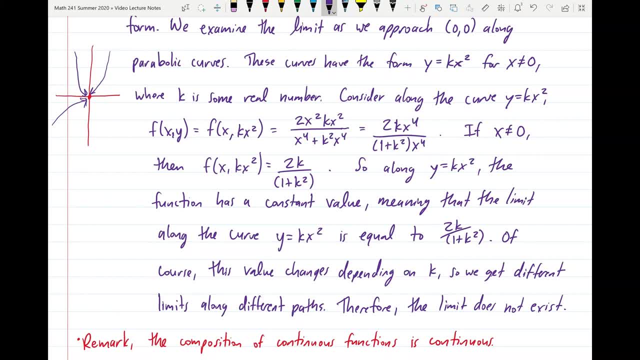 origin. so we're going towards 0: 0.. so we're going towards 0: 0.. so we're going towards 0: 0.. um, and so we can cancel this x to the fourth on the top and the x to the fourth on the bottom. 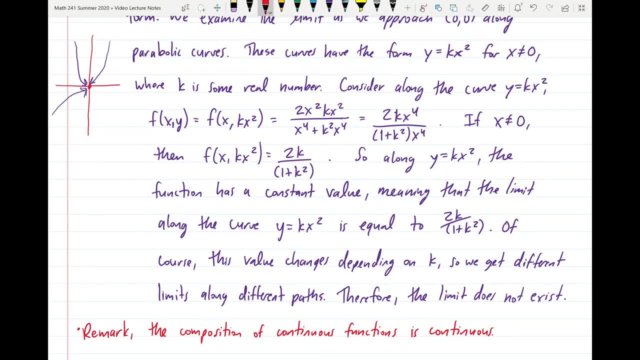 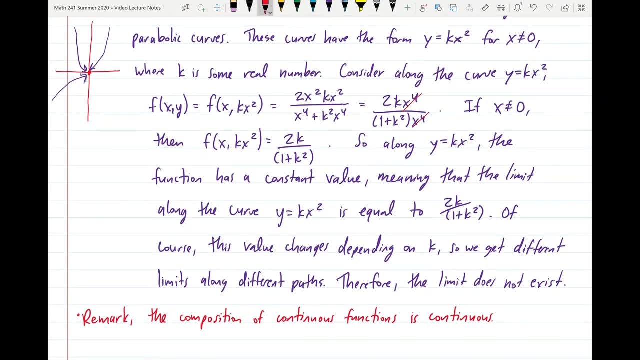 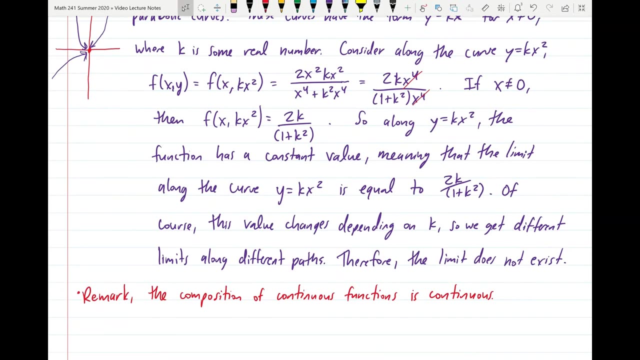 that shows up in our function here. let me just draw that so we can cancel these two x to the fourths. and so the function f of x, k, x squared ends up just equaling 2 times k divided by 1 plus k squared. and so, along the parabola, y equals k, x squared. the function has: 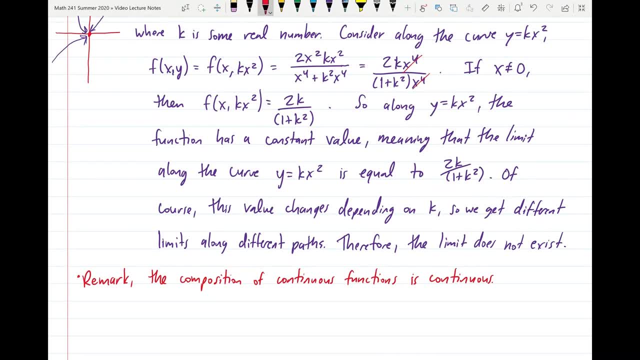 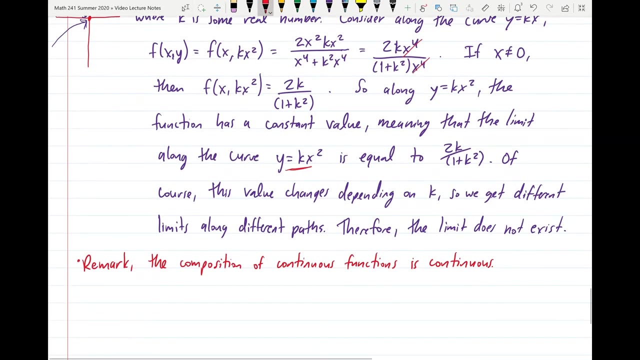 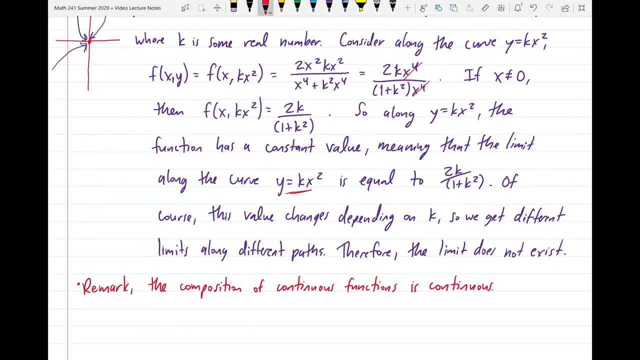 a constant value, namely 2 k divided by 1 plus k squared, meaning that the limit along the curve y equals k. x squared is equal to 2 k divided by 1 plus k squared, and of course this value is going to change depending on what k we choose. so we can just choose um two arbitrary parabolas. 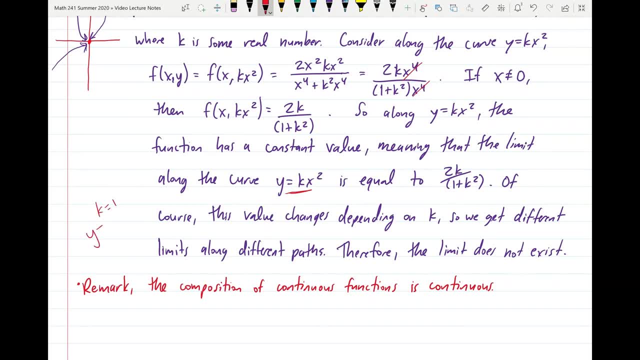 say, we choose the one where k equals 1, so that equals x squared, and then we can choose the one where k equals 2, so that y equals 2x squared. and if we approach the origin along these two different curves, then we get different limiting values and because of, because of the theorem, 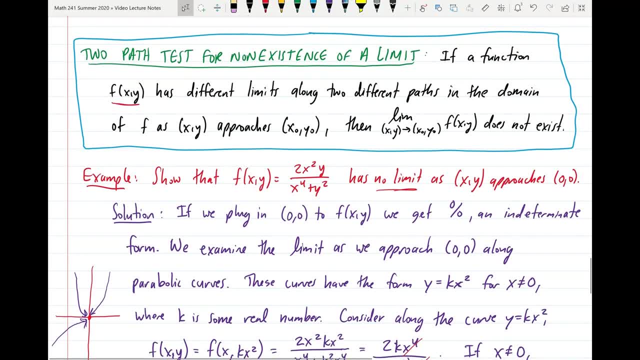 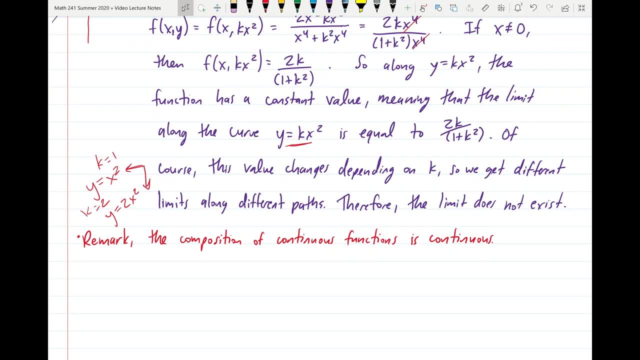 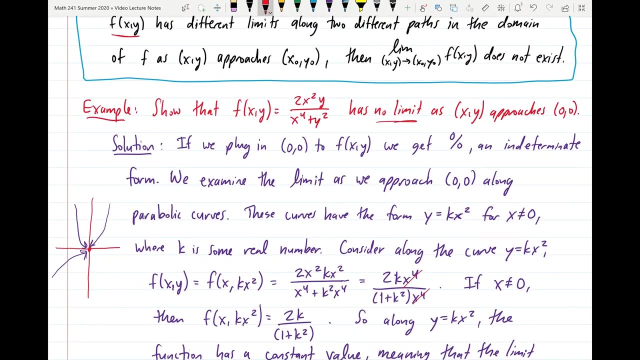 that we have, above this, two path test for the non-existence of a limit, because we get two different limiting values as we approach along different paths. it implies that the limit at the origin does not exist. so we can, we can conclude that the limit of our function as we approach the origin doesn't exist, and I 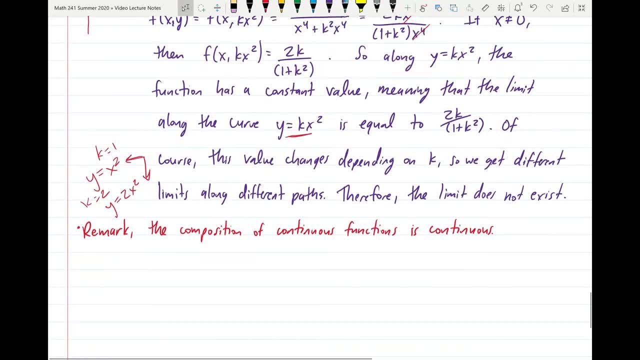 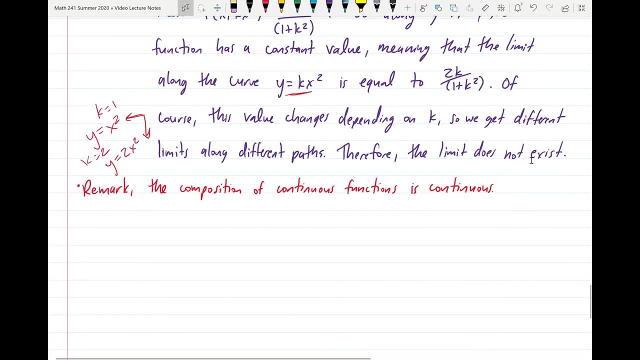 will give a homework problem, at least one of them, where you're going to use the, the two path test like this as well. so the last thing for this section. I just want to give a remark, and that remark is that the composition of continuous function is not constant. 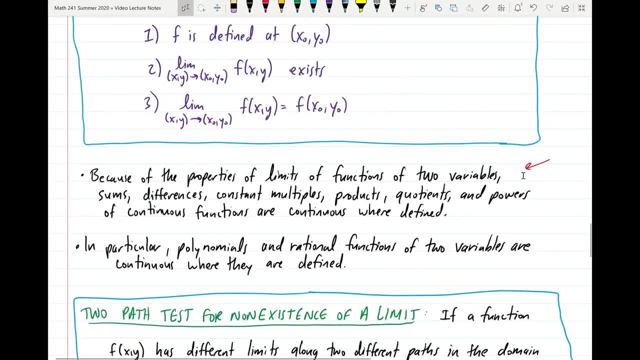 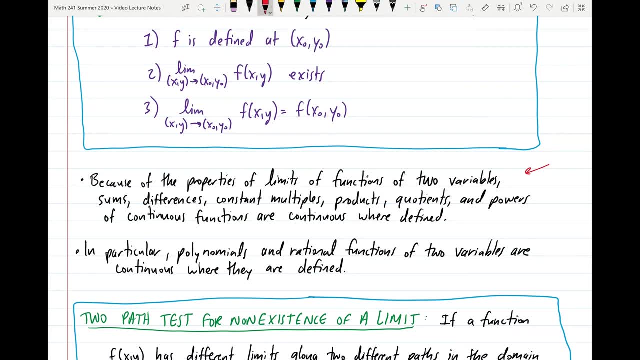 so may I just give you a very brief answer. so I remember before when I earlier called it continuous, so CONTINUOUS, which is accordingly an expression of possible present lives. and we're talking just about what continuous functions are, and I'll explain here what continuous functions. 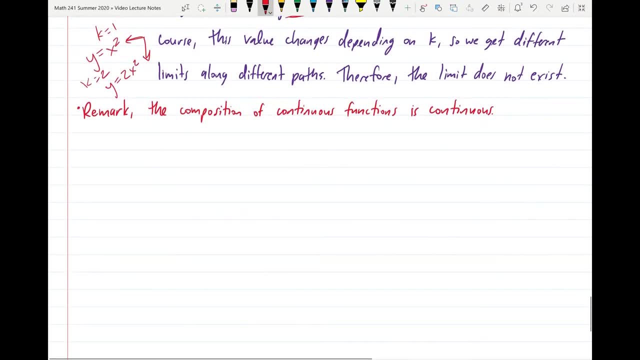 are. and then, final point, we'll go from right now. so contiguous functions, test I'm called. continuous functions on n1 are continuous and somatic functions on n2 are not continuous. SUBC documentation is not, but there is two. seems to be some干alog here about continuous functions, and continuous application brings us to the form SUBC codes within our exhibition.